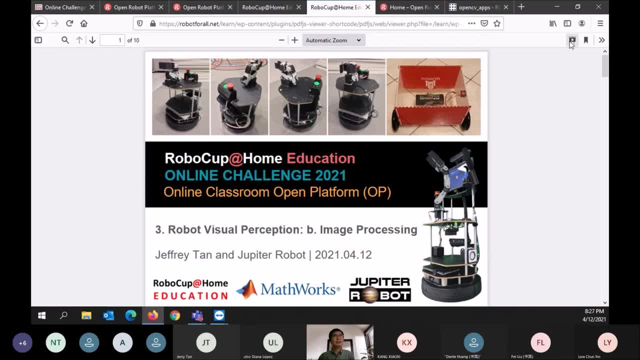 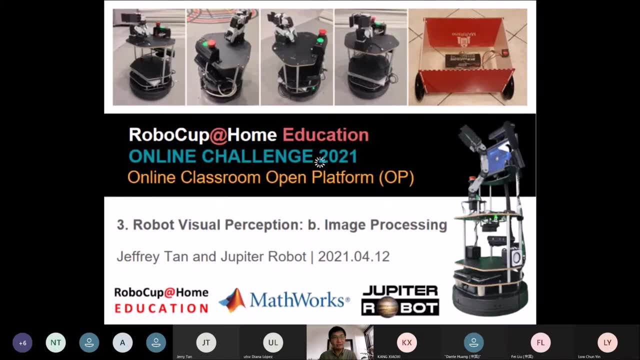 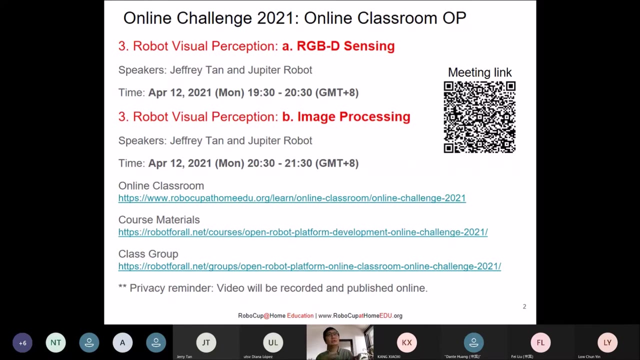 Right, Okay. So for the second part, we will talk about this image processing, And now I'm going to like tell you some of the theory part. then I will pass to our colleague in Jupyter robot to show you the actual example. Okay, But before that, let's start with the introduction. Okay, So I will skip this. So, basically, now we go to the second part that we are going to discuss about this image processing. 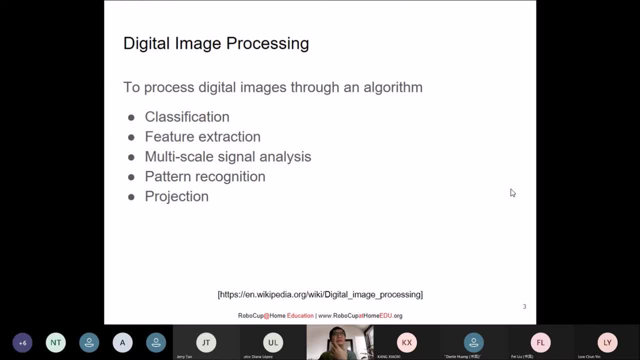 Okay, So for image processing, digital image processing actually is a process to process digital images through an algorithm. Okay, An algorithm can be a mass algorithm and so on, Because you know, digital images actually are array of figures, Okay, Data, or like value. RGB, basically, is 0 to 2.. 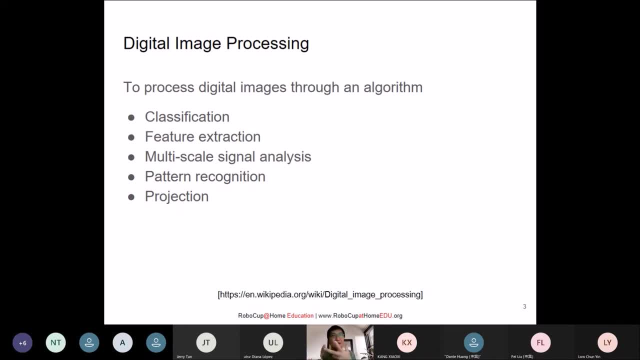 0 to 255 for R, for G, for B, So you got like three value And then you have the whole picture for all the pixel. So you have a big array of numbers. So these numbers it actually give you a certain pattern And also by applying mathematical algorithm to this array, then you can actually do some analysis and also do some processing to obtain certain objective. And this 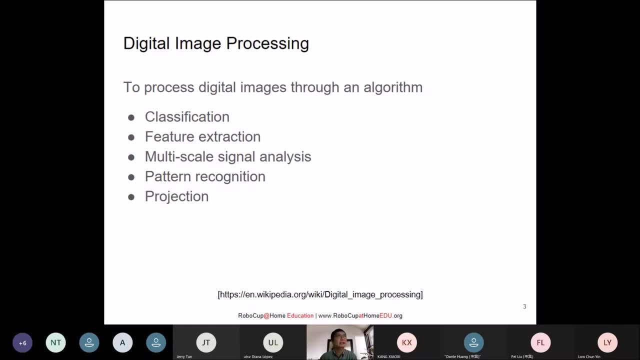 whole process is what we call the image processing. Okay, And there are, there are many application for this image processing. like classification- you can classify different thing. features extraction- you can extract, for example. like the way how we actually recognize certain thing or certain track, certain object in a photo is like using the features extraction. So we extract certain features and then we track the features and so on. 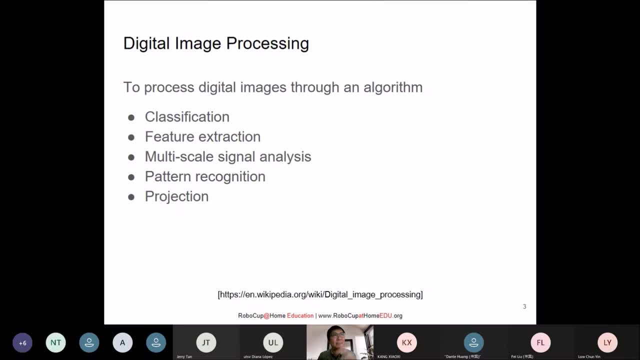 Then we have other things, for example a multi scale signal analysis and pattern recognition. Yes, pattern recognition we use a lot, Okay, use a lot to find certain patterns, for example how you find the outline and so on. So those are pattern recognition, Okay. so there are many techniques, projection and so on. Okay, so you can go to like Wikipedia page and see like what are those by a lot, Okay. Okay, but for this class we are not going to talk a lot in the theory like how is the algorithm, how you do it, but we will straight away talk about the algorithm. 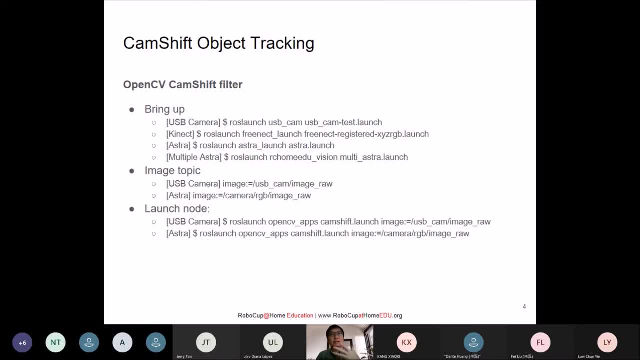 it away, show you, like how to do some example of some application. Okay, then you will have some idea like how to use this thing to develop your application. Okay, so there are a few things like. I will just introduce you this, So later on I'll pass to engineer Jupiter robot to show you the example. So the first example that we show you is the open CV cam sheet filter. So this is one of the example in. 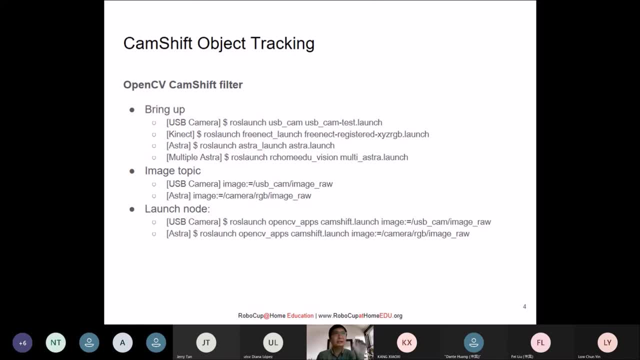 the ROS open CV application library that I just introduced just now. So the procedure is like you need to bring up your sensor, So you need to get the sensor ready, then you need to know your image topic. Okay, because different sensor when you run the driver it will give you like it will actually like fit the data into a particular data topic. So for the USB camera, the topic is this: USB underscore cam image topic. 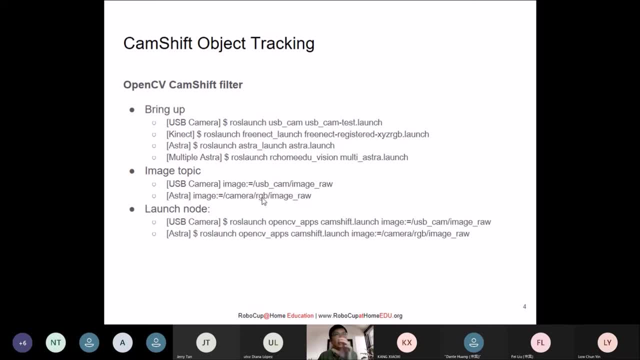 And for Austria, the RGB, the RGB data is fit into this camera. RGB image raw topic. Okay, and you can find more topic once you launch the sensor. Okay, so in order to launch this cam shift node, this is how you need to do for USB camera. So you launch it like the cam shift. then you need to specify where is your image topic, or which one is your image topic. 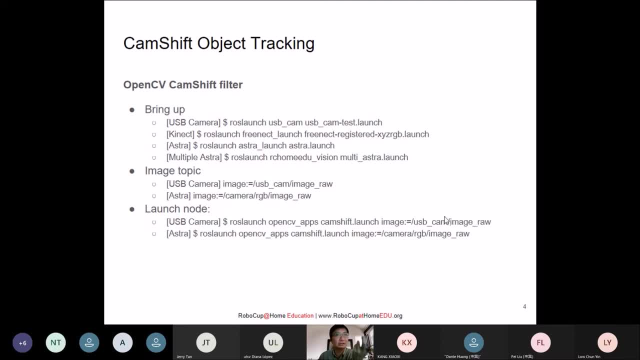 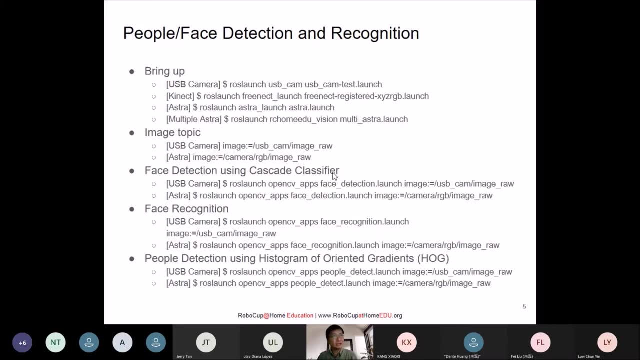 So you specify over here. So this is the difference between these two. Okay, so then we have the face detection, which is the same procedure you bring up. then you use the image topic to launch, for example, the face detection using the cascaded classifier or face recognition, or people detection, and so on. Okay, so these are a few examples that I would like to introduce our colleague in Jupiter robot to show you the image topic. 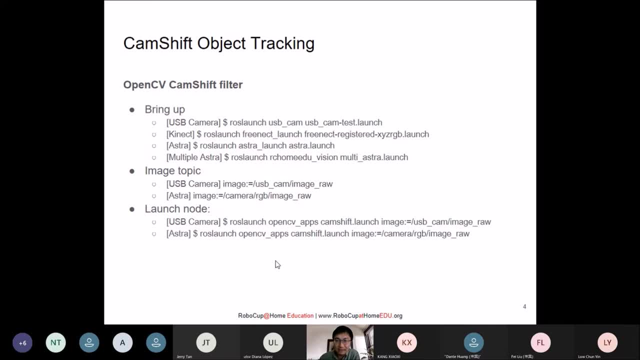 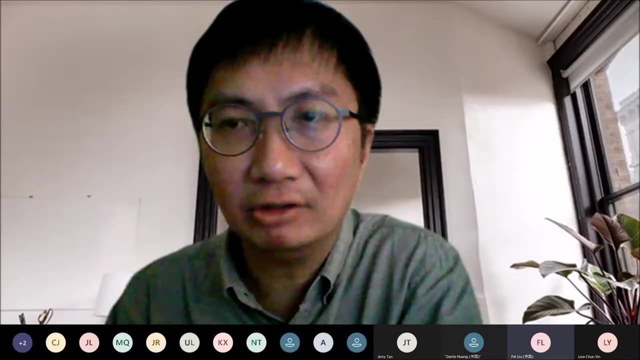 the example. Okay, so may I introduce some? David? Yes, I'm here. Okay, so I'll pass the screen to you and please show us the example. I will share my screen. Okay, Can you see the screen? Not yet. 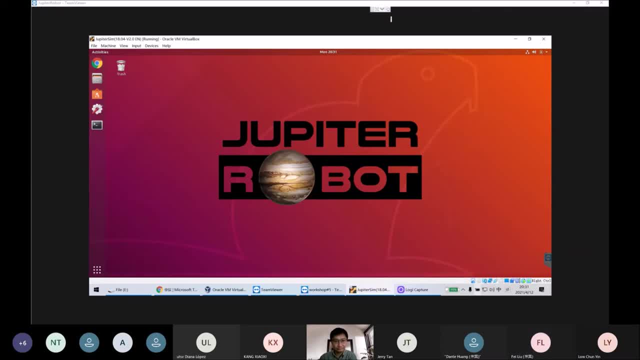 How about now? I'm still waiting. Maybe my site is a bit lagged. Yes, I can see. So you can see the virtual virtual box. Uh, virtual machine software, which is a computer theme, Is that? yes, Okay, yes, I will start the demo First time. you show you how to connect your USB camera to the 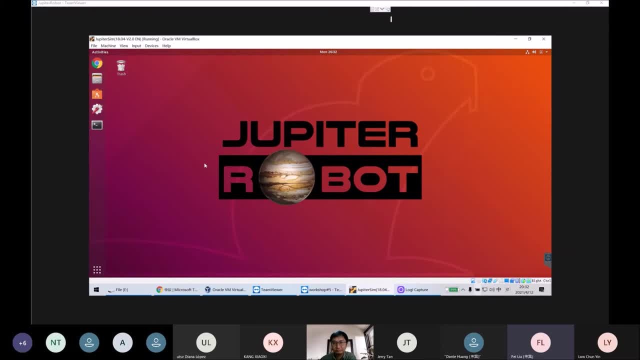 Jupiter steam, which are box virtual machine, which means if you use the virtual box software you'll need to mount your Uh device to the stuff, Uh to this virtual machine. Uh, for example, we also we always use some Input device such as aasonicphone on the speaker for the sound to connect with. 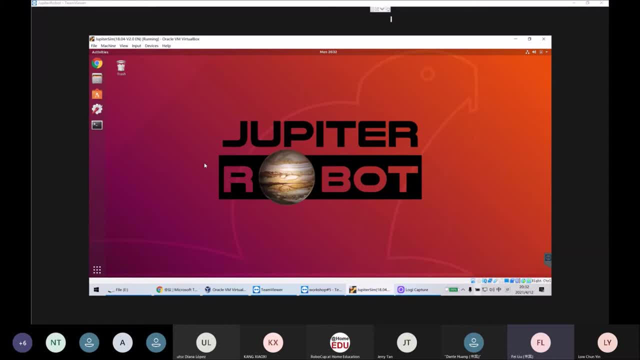 Uh, virtual box, and now I will introduce how to input the camera. Please pay attention to this button device. A�pren, select the USB USB. There is a list of all your ah. connect to USB interface and the camera is properly connected. Please see this button device. 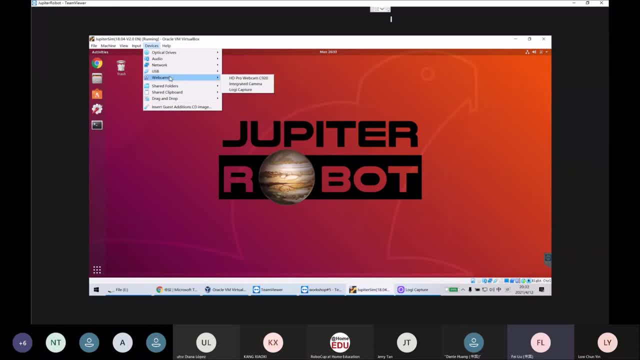 interface device. There is also a webcam list, but I suggest we use USB to connect the USB camera. I think most people who use a laptop they have their own built-in camera, but I suggest you connect another one, especially for USB camera, to the computer or your laptop, because 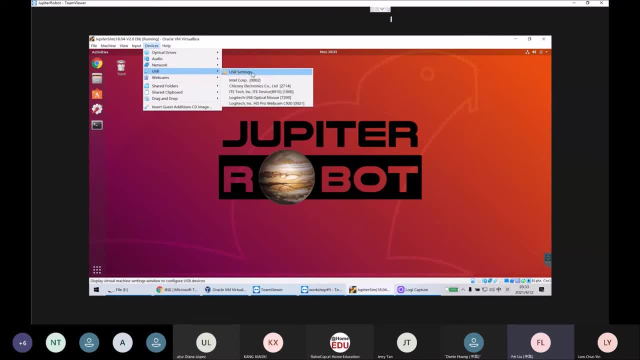 this is easy for the virtual box to know the interface of USB camera. So for me I have an interface with Logitech, Logitech HD Pro Webcam C920.. So I click here. you can check. now there is a mark behind this camera, So this means I have. 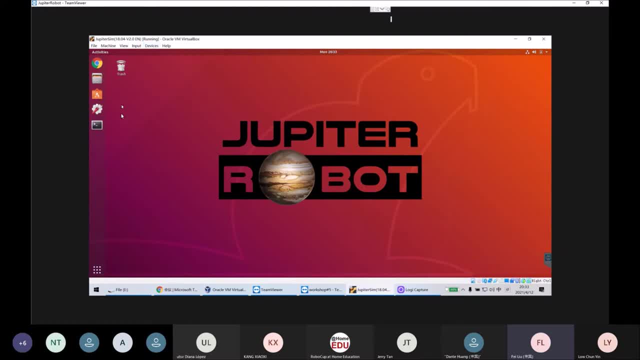 a webcam. So I click here you can check. now there is a mark behind this camera. So this means I have a webcam. So this means I have a already connected the camera to the virtual machine. So now I will start to launch the USB camera. As you can see in the PowerPoint, we can use. 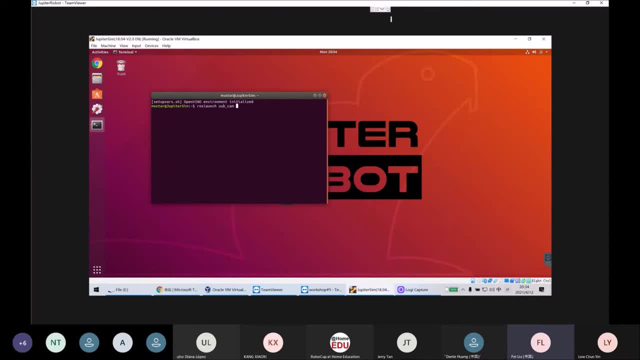 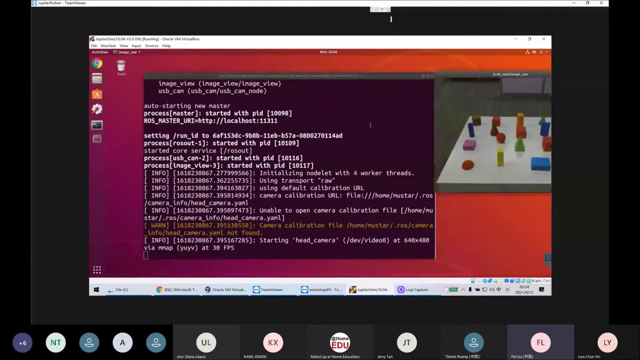 useLaunchUSBCam. This is a package name and the USB. you can use a tap to auto connect to the left part of the command. We can use this command to launch up to 8 inputs. sorry, This is much better and this will launch the camera. Okay, this is a camera. this is. 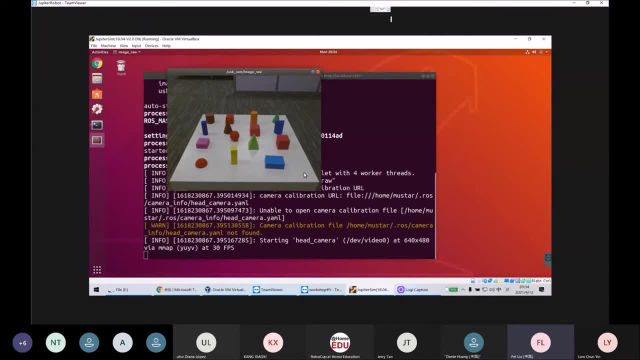 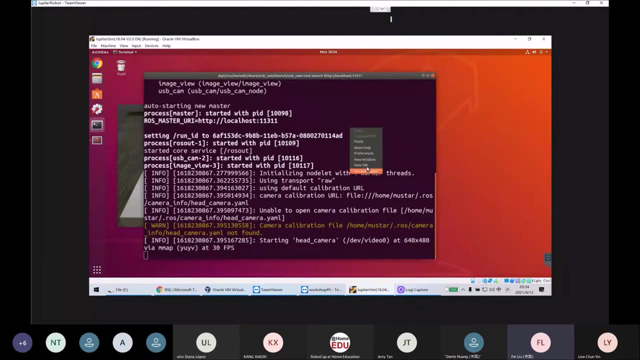 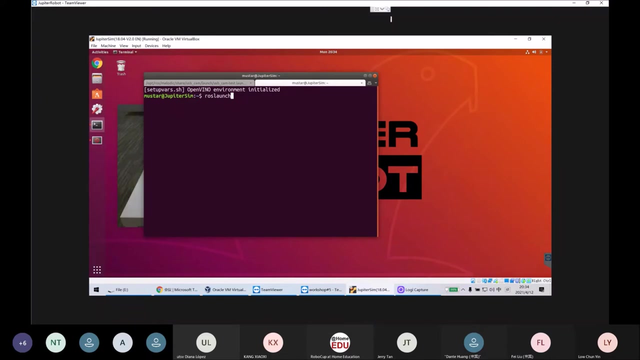 the image camera captured by the camera to show you this demo. And this window is just to show the image of the camera. it's not the processing procedure of this camera shift, and now i will open another one. first, launch open cv apps which have already building the uh package. filter a photo: uh here. 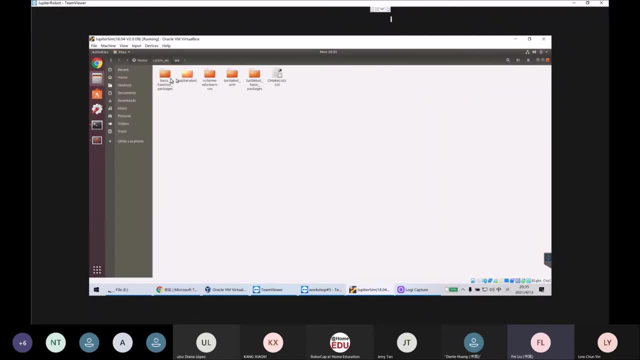 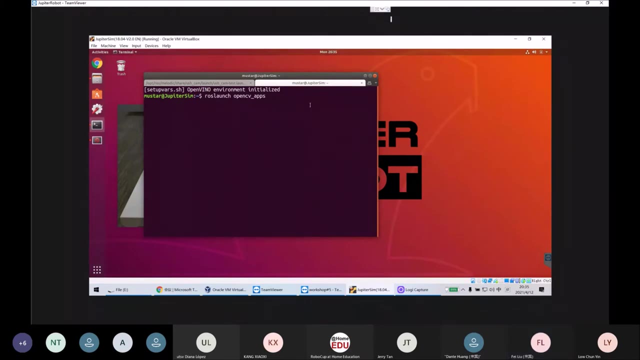 i can show you cat king workspace, src basic function, basic function packages and here open cv apps. we have already building this source source code package here. okay, and cam shift- uh, we also need. we also need to specify the topic, you might. oh, i've almost forgotten the topic and i will check this one. 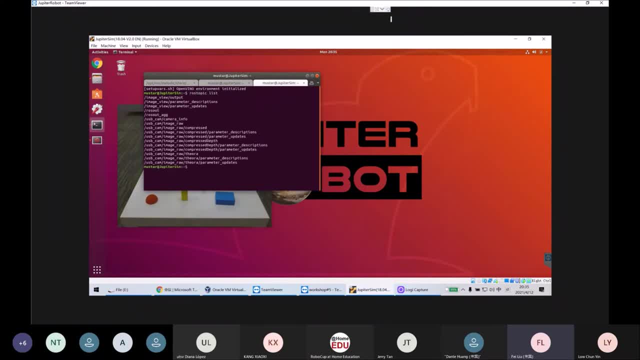 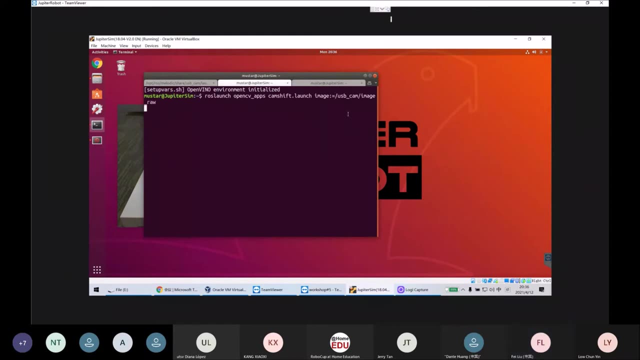 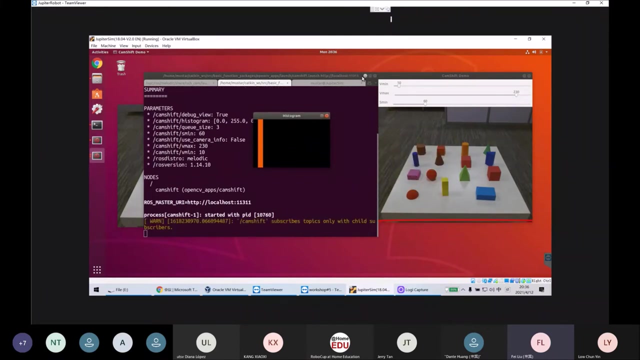 rose topic list we can find that the image image for this usb cam is here. we can copy right click and then copy here. past. okay, uh, we have uh open two windows. uh for this demo. here is a histogram for the uh cam shift. uh cam shift demo. use h, s, v color, space for the color. specify and tracking. and. 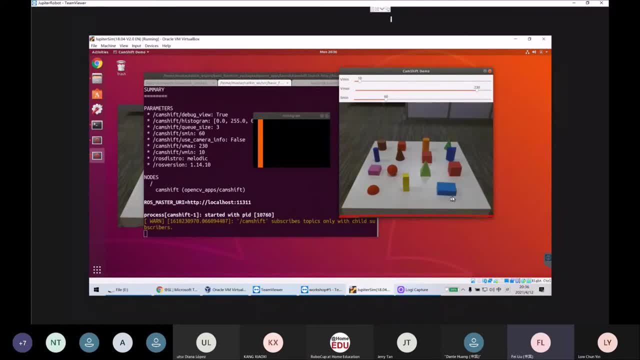 uh, i will show, show you if we want to track this one, for example, this uh light blue, i will left click on this object and uh drag uh ship. this will select the each value of this light blue uh object and uh, i want my, uh, my partner to pick up this one and uh move in this in the field of the camera. 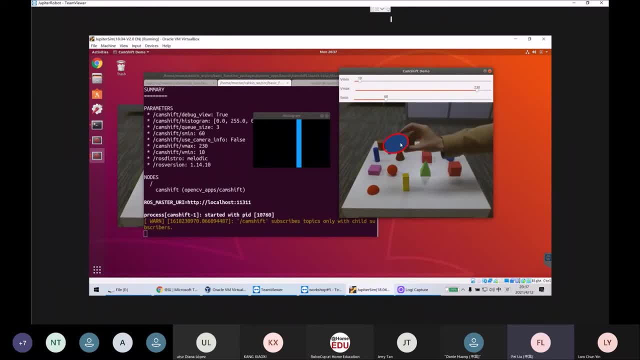 you can see that the camera shift tracks the object very, very good and uh, now, uh, but i'll not have to go if we leave this one and then the cam sheet, we will select the most uh, most most uh similar one, for example: this is a little. 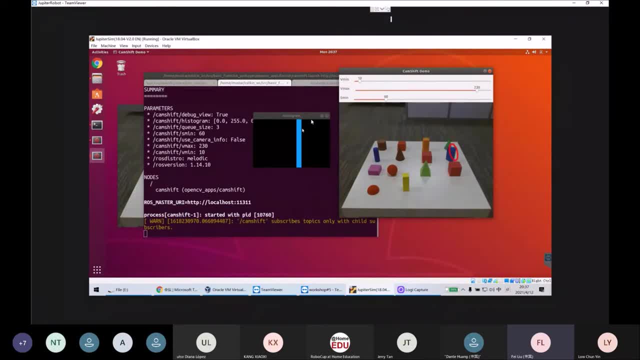 dark blue. so if we don't have this light blue, this the- the cam sheet view- tracks the light blue. so if you want to track this light blue again, you need to put this glue near to this and that we will check this one again. So there is also some value we can adjust to. 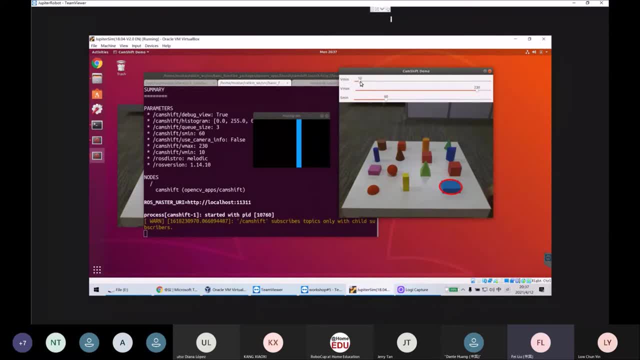 inflect the effect of this camshaft. So we have three thresholds, which means the light value of this object, mean value and the V max is the max value of this object. So if we drag the mean value to be larger we will find that maybe at some position we will not lose the 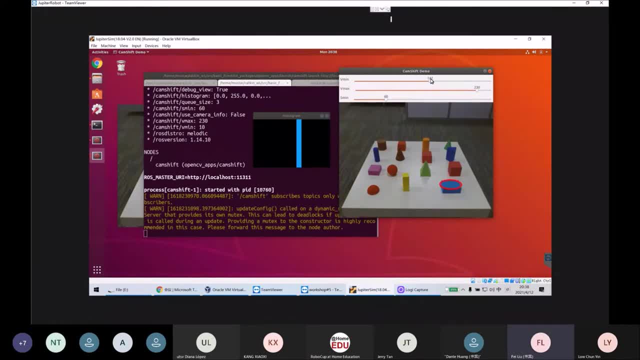 track result, because this mean, which means that the light value of this object is larger than the wing mean and the smaller than the be max. Okay. And X means the certitude of this color. So it's also we can use this value to make it more specified. Set this value to track the object, Okay. So this is a kind 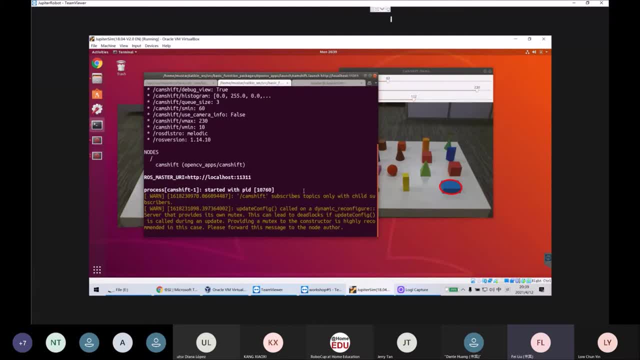 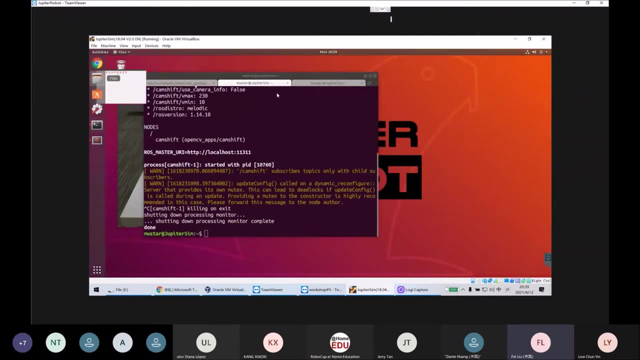 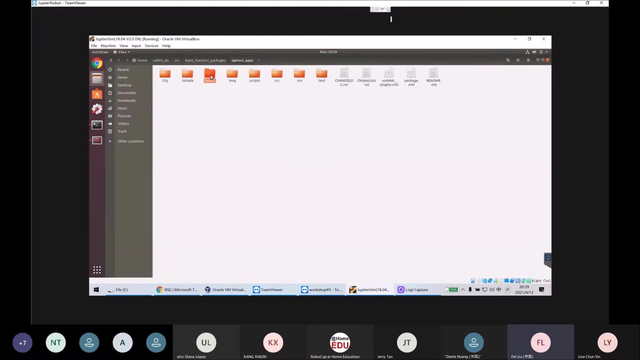 of shift, And I will also use this sample to show another result or another example In this photo, for example, of MPPs. as you see in the wiki, we have all this package here, I mean this launch file. You can find all the launch files And I will show you. 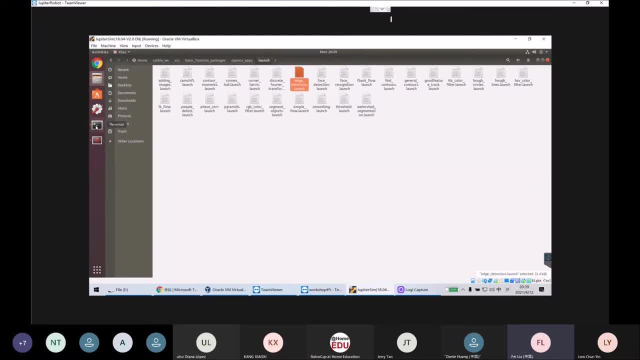 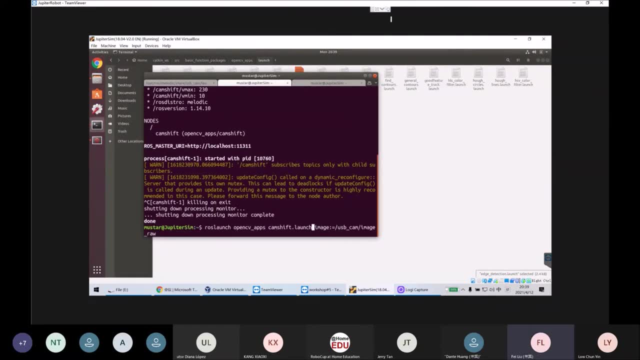 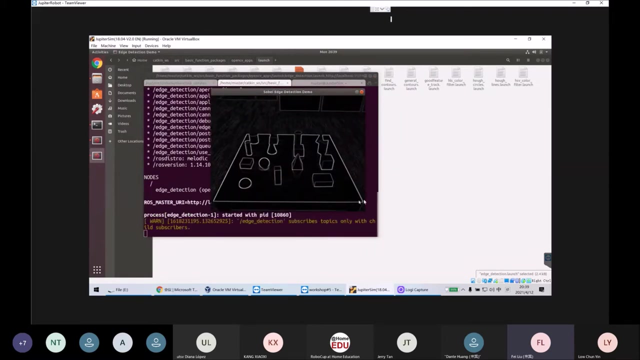 this one Edge detection: Edge detection to show the edge detection result of the object. So I will change this. this launch file Edge detection launch And then it will show you the edge detection result of the object. This is almost the perfect edge detection because it's smart and single. 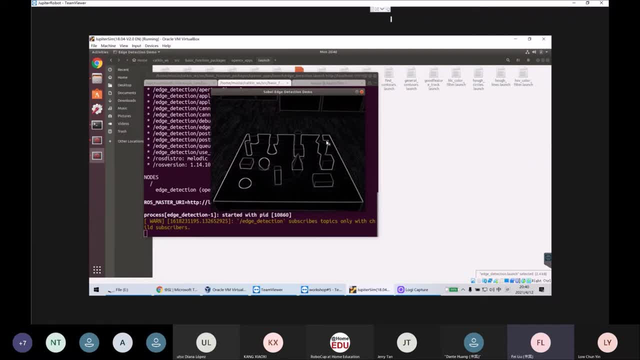 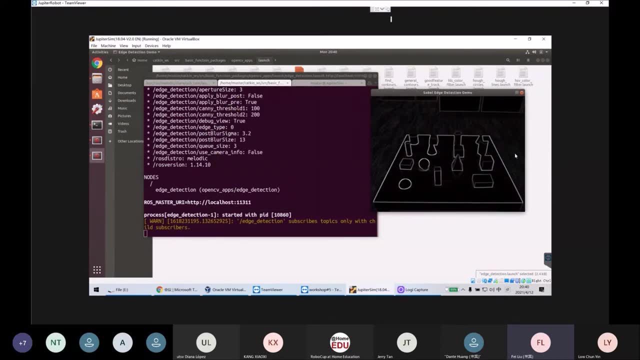 pixel, pixel edge of the of each object. We can also show you the Oh. sorry, I will let my partner to show you the uh, yes, real time, real time processing result of edge detection. I can see. it's very good for the edge detector. Thank you, Okay, This. 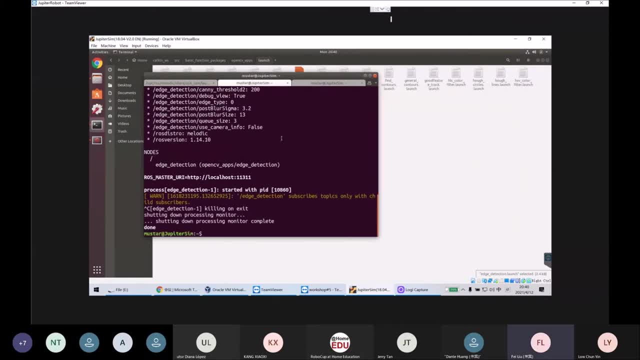 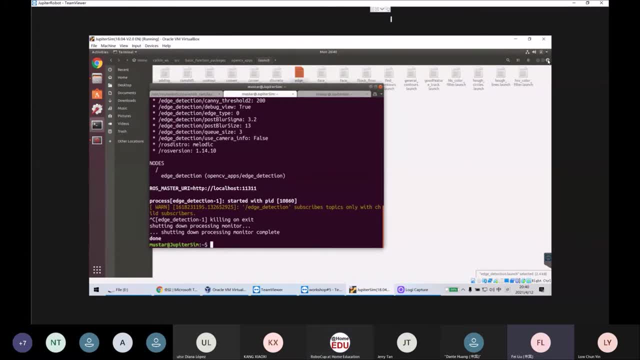 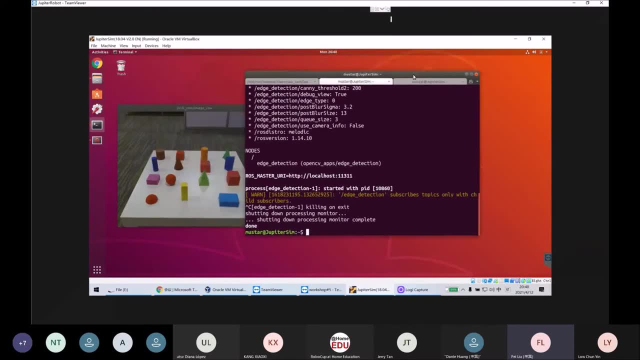 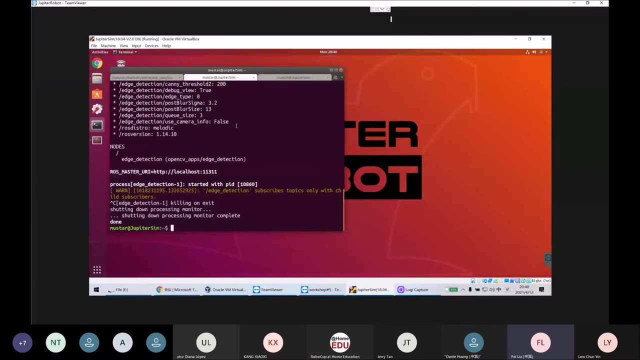 Okay, And now I will show you the face detection and the face recognition and the people detention. I Will. So, for your, for the Face detection, I will- Uh, I will use this one: Rose, launch open OpenCVAppsFace. 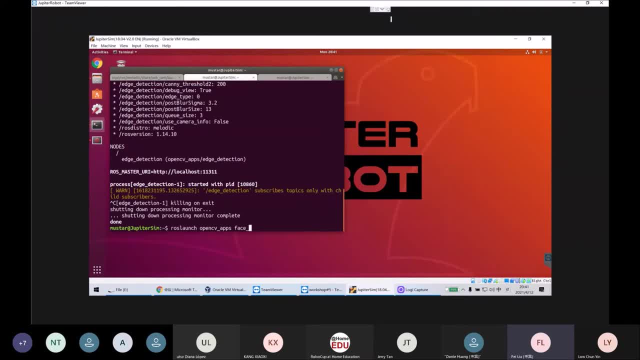 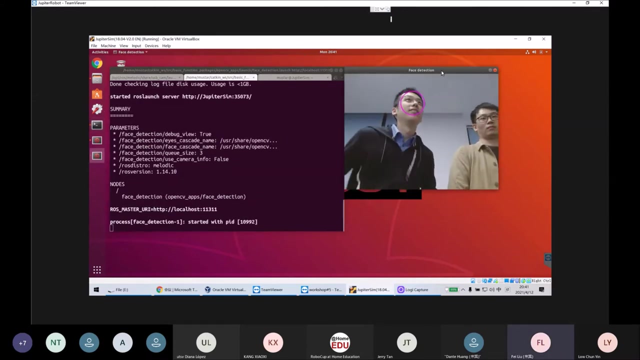 So for the face recognition, the first procedure is to recognize the detection, sorry, detect the face in the image. So I will show you first the demo face detection launch and also we needed to specify the topic also. They are my partner. 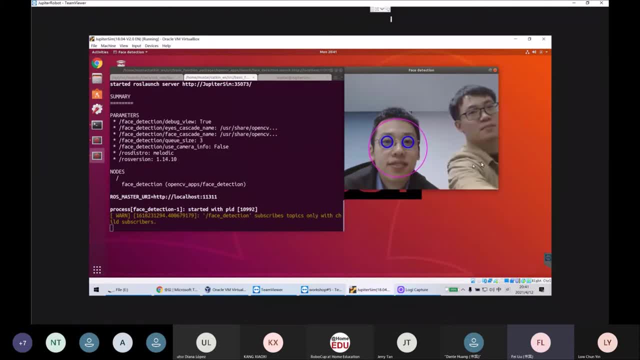 of the robot and then you have one, and then you have one. So you can see the face detection result in the demo window. So, face detection: this circle, purple circle, will show you the results of the detection of face. So we have two face here. 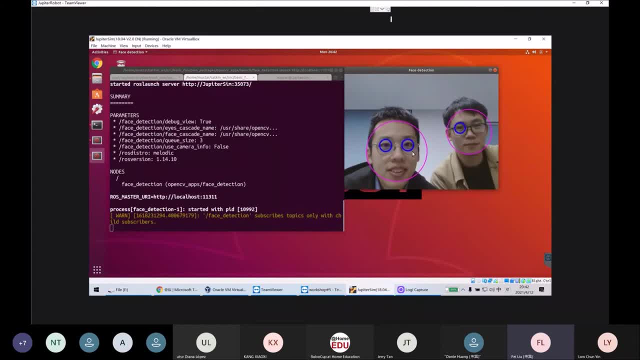 we have two circle and this blue circle means it detects the position of eyes. Maybe sometime you can see the detection of the mounds. So this is the result of face detection. But most important application for the face detection is to recognize who is who. 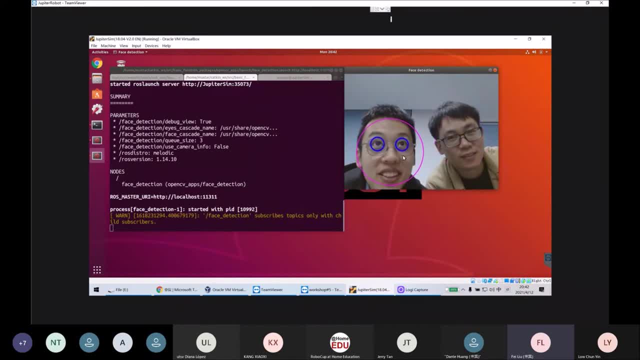 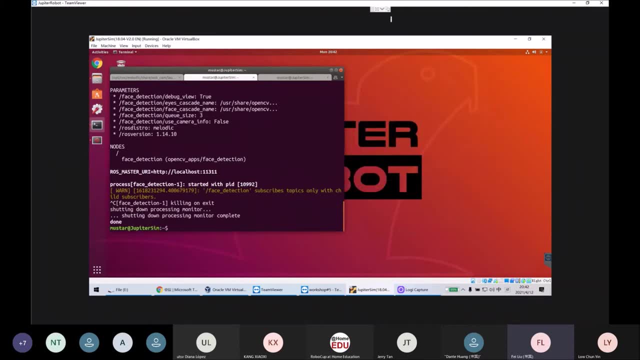 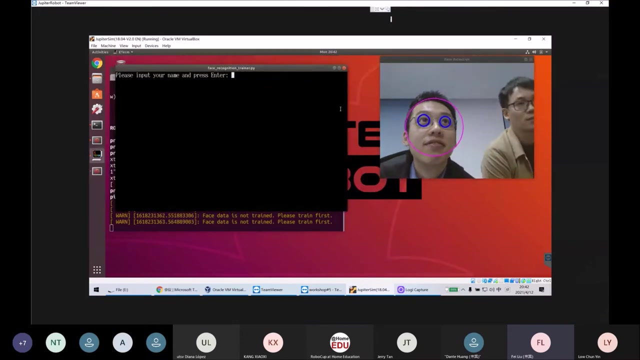 I mean recognize the people in the image and mark the name of it. So I will show you another demo which means: which is the face recognition? Okay, There is a window here, So just the one in the image. So I will tell the program who is it. 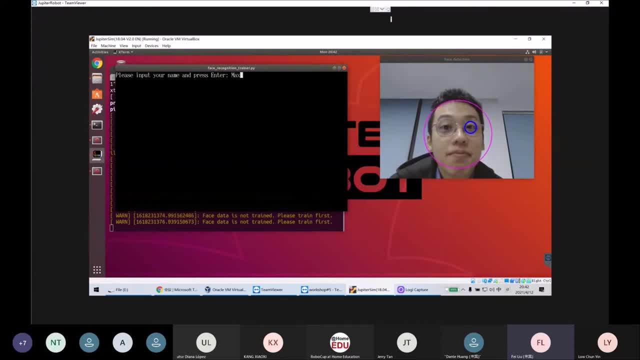 Who is he Name? Max. I type the name of Max And the program asks me: is that correct? Of course yes, And please stand at the center of the camera and press enter, which means we will start to take pictures for training the program to know he is Max. 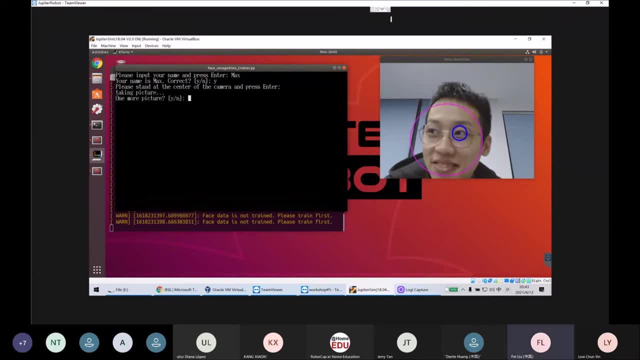 Okay, Thank you. First, if we want to recognize a person very well, I mean for different condition, we needed to take more pictures, And we will take pictures about five to 10.. So I need to ask- I didn't know who- to show different side of his face. 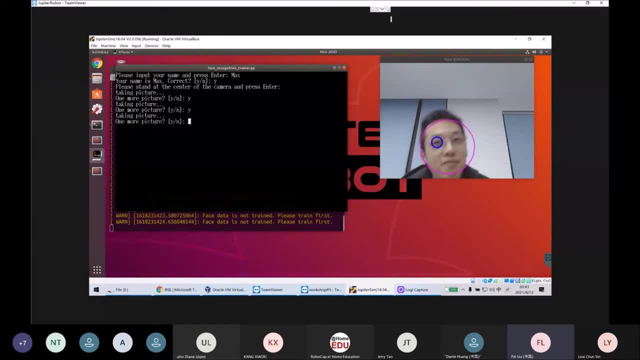 Okay, Well, I'm sorry, Call, Hold it. Sorry, Call, Hold it. They did, I got it. I got it. Okay, Okay, And and uh, go to see if we're going to tell me. 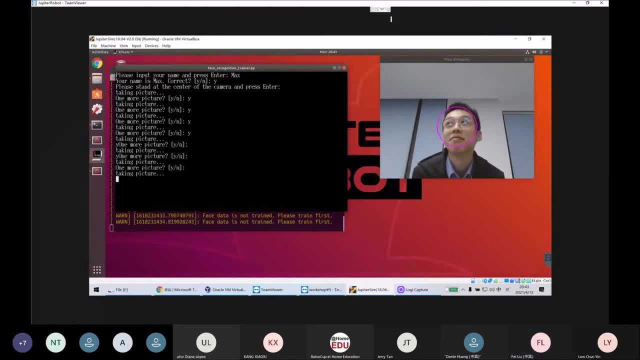 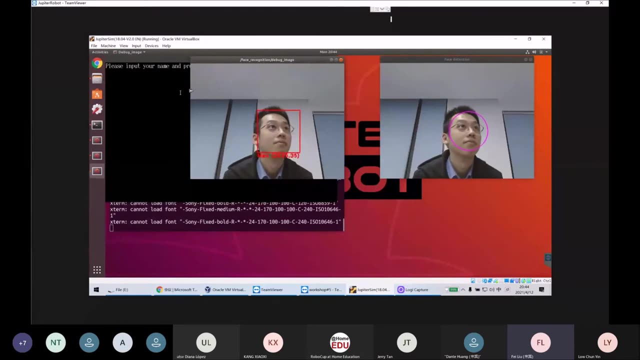 Okay, Very well. So if you think it's enough for your training, you can tap no, which means it's over for the training, Okay, And then it will start another window to show you the recognition result, which you can see here. 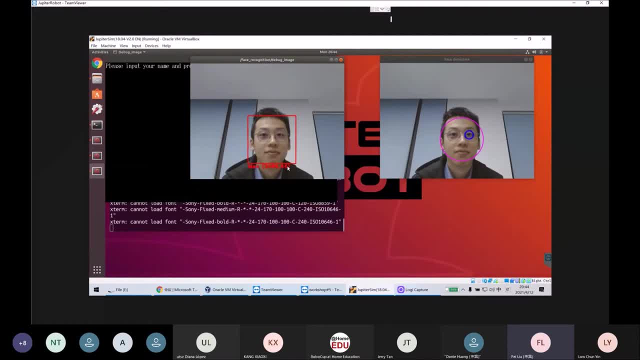 Max, And this value means that the program think the reality of this uh recognition result. So could you please ask engineer Huang here to show the uh deep tool base here? Okay, Oh, you look. uh, they look very similar. 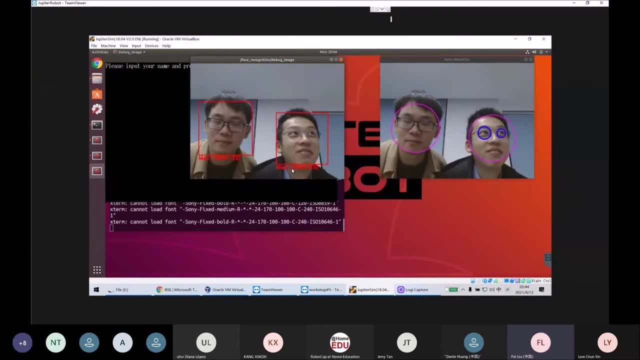 So this is the right P? uh. people face recognition. So this is a based on the people face uh detection here And uh. this is the result of the people uh recognition. So if you want to uh. 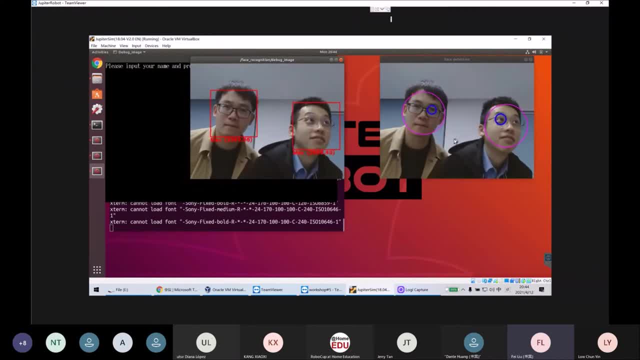 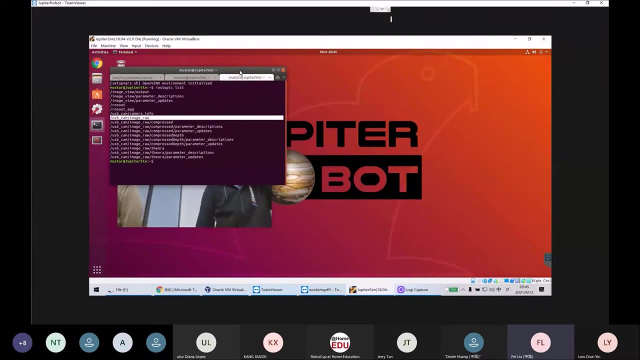 detect the people very well. I think you need to train more pictures to let the program know who is who. Okay, Thank you, You'll shut down this program and uh, uh, how the the the profile, uh, how the program know the. 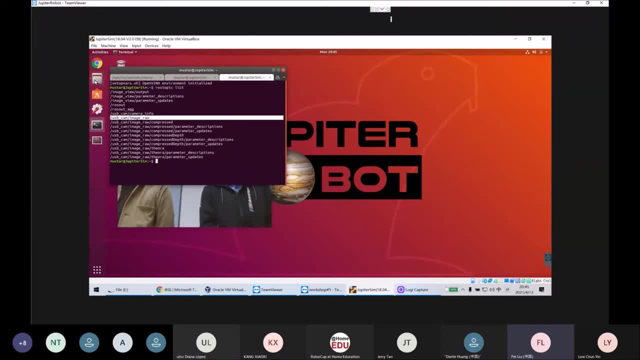 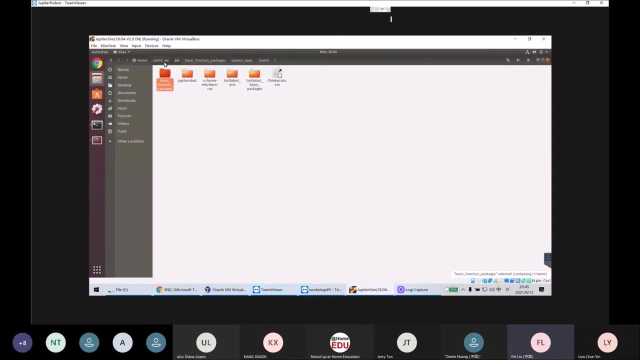 uh, how to training, how, how the program training the result they need to start, uh, uh, uh. sample image in the uh computer. So I will show you where the computer, where the rows start uh. 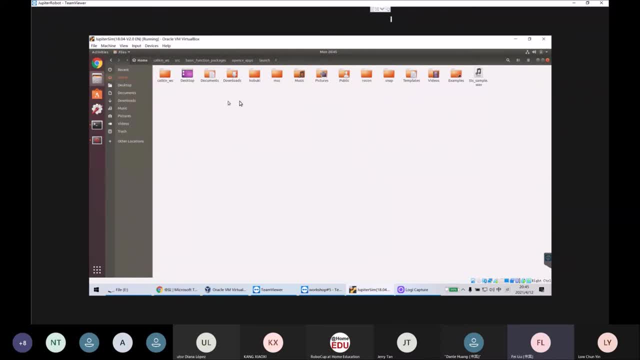 uh sample image. So at this uh home photo, uh, you can press control plus H to show you the hidden photo, And here dot rows and you can find uh open CV APPs. Uh and uh. 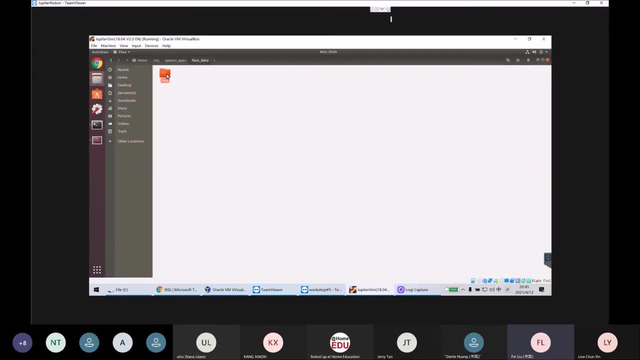 face that the name of the person you need to detection detect And this is the image we just take for training the program to know who is Max. So if you want to uh reset the detection result, you can just uh the delete Max folder and the program view not know who is Max. 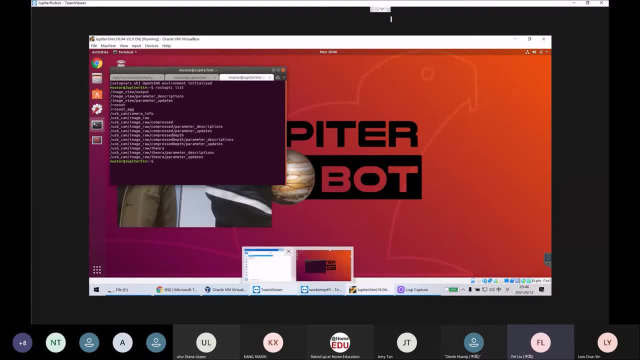 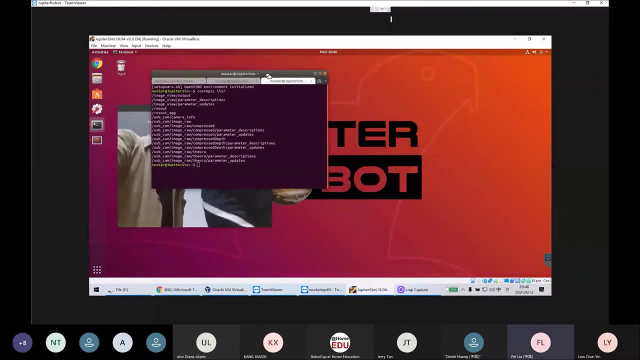 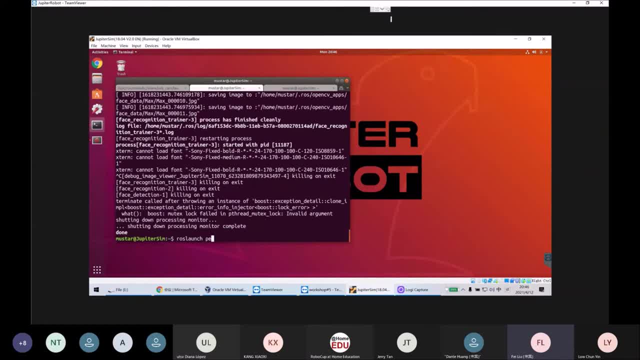 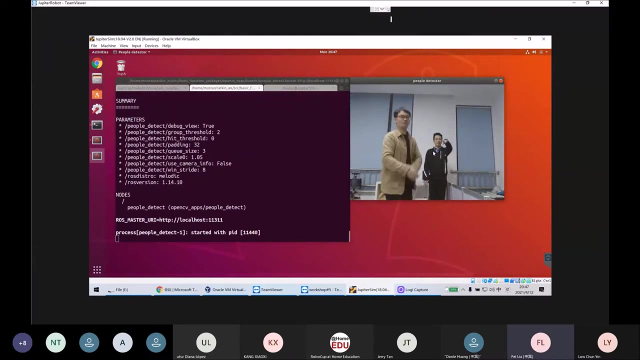 Slam ch P P Pro. uh, sorry, I forgot the package name, Oh Detection, and also needed to specify the topic. Nothing Uh The people detection need to see. Uh a little OK to see the whole people In the image. Nina has to do this. already made it. 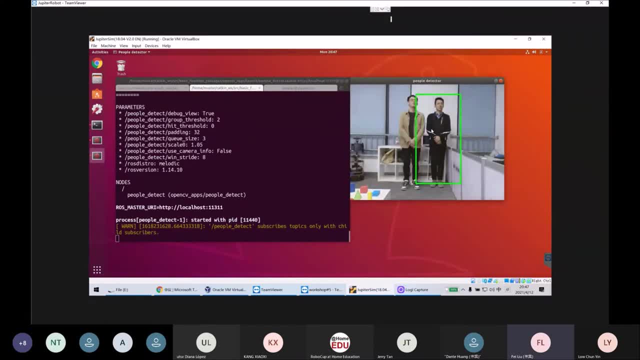 Yes, uh, it can detect not only one person, maybe several, several person. I, which we have a train, have tested more than three person is also OK. So I think Max is a better than the underneath one because he's have a white Background and the black Black, uh, close. 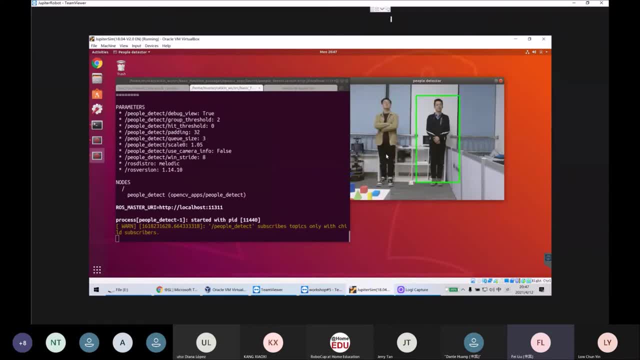 It's much better than the one to show the difference, uh, between here and the background. So this is the result of people detection. OK, thank you so very much. Now I'm in a country. So, Professor Jeffrey, can we show you the? 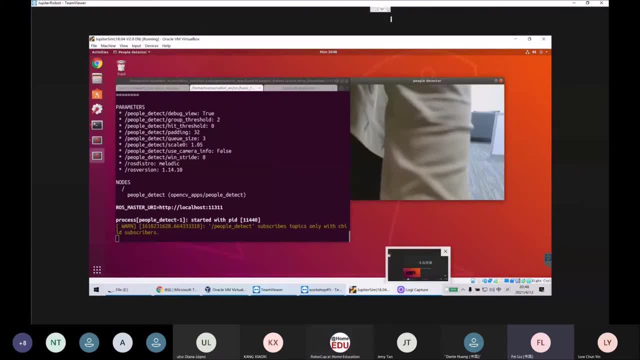 So you need that, you need need them as to show you the tracking and which means follow. OK, can you show after after Pardon, you show after after explain? I mean we next we will show you the result of demo of follow. So we need, we show follow on. 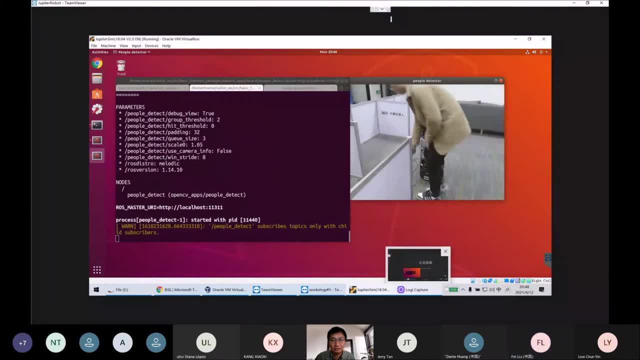 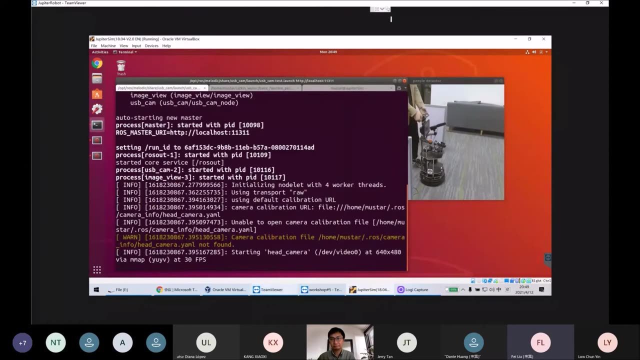 I can't hear you. I can't hear you. Uh, wait, let me. Let me explain first, then I'll pass back to you. OK, thank you. I see, Uh, I will stop Share my screen, OK, thank you. 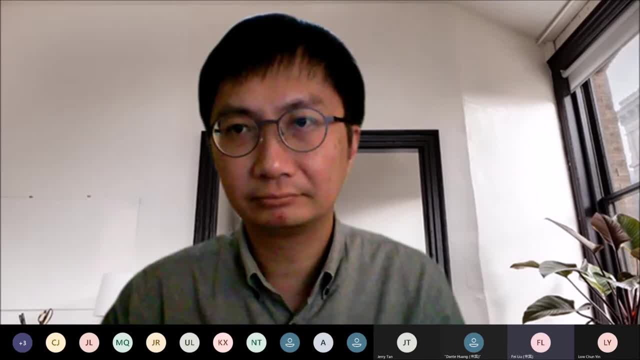 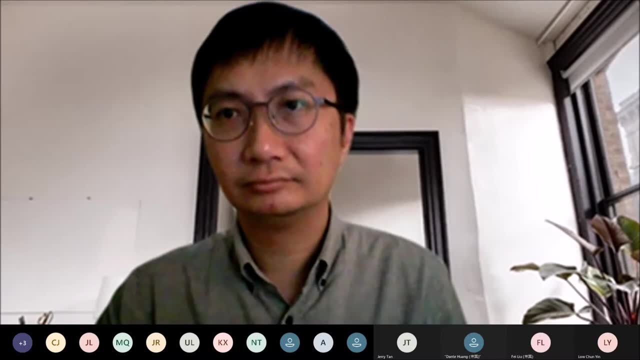 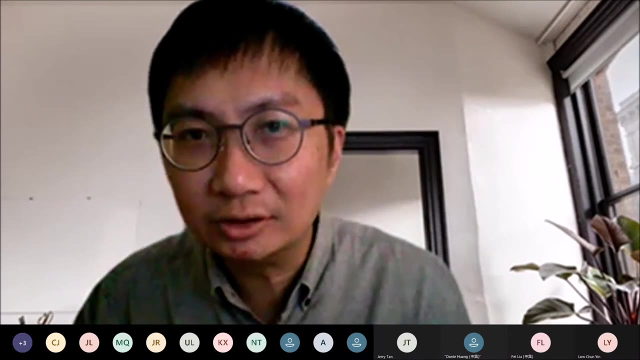 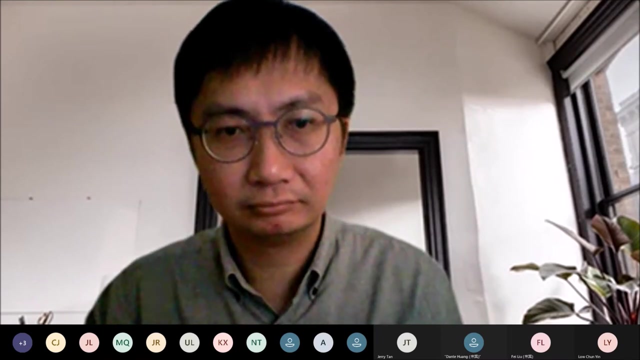 It's your turn. OK, That's OK. Yeah, yeah, I'm going to take a picture, OK, OK, it's uh, it's quite heavy over here, So give me some time, OK, OK, So I'm going to do my tests. 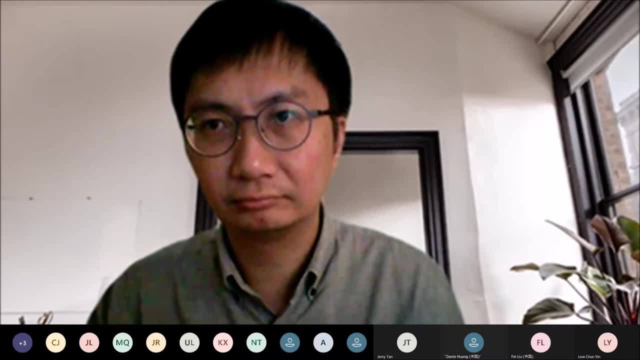 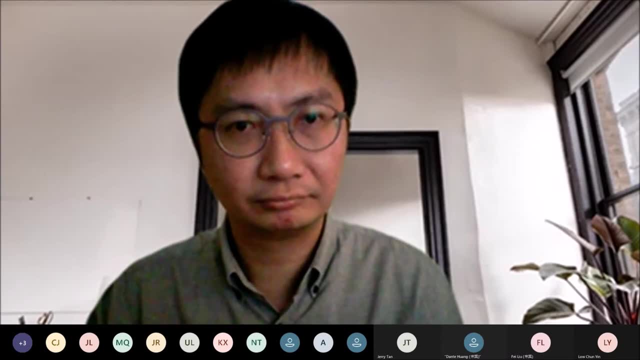 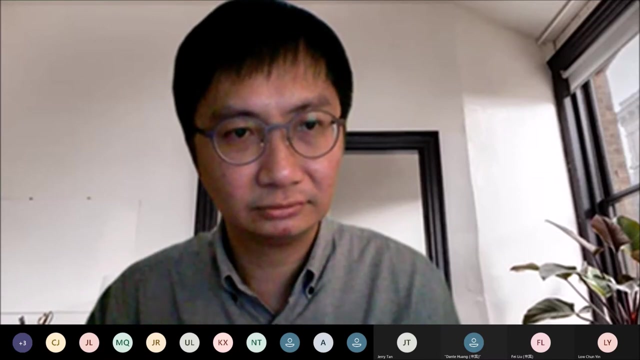 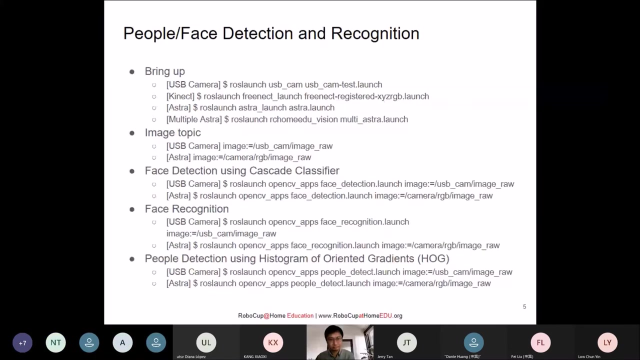 OK, so I'm going to see if I can see the forks. OK, it is OK, OK, OK, OK, OK, OK. Thank you, I hope you can see my screen now. Hopefully it's okay. Okay, right, So just let me add something. 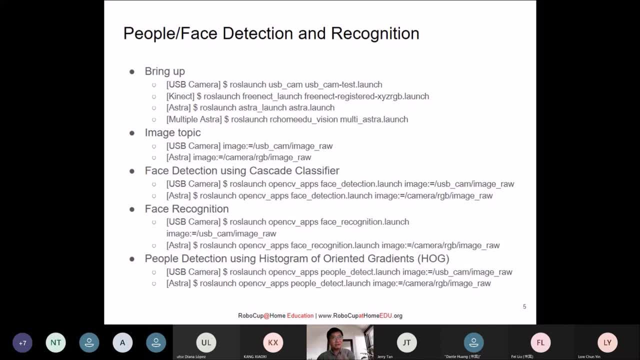 For the demonstration just now. So first of all, thanks a lot. Thanks, David Wu and Huang, for the demonstration. So I believe now you have some idea how to actually use the OpenCV APP library, So it is very useful for you to learn how to use that. 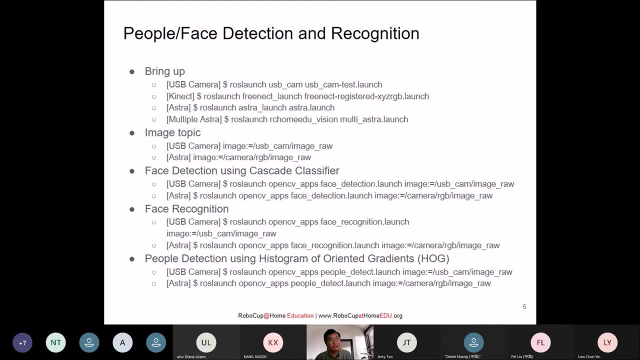 Because you don't need to actually start from scratch to write your OpenCV code for your application. You don't need to use the object recognition or something, because it's already packaged nicely, But you need to know how to use it. Okay, you need to know how to use that. 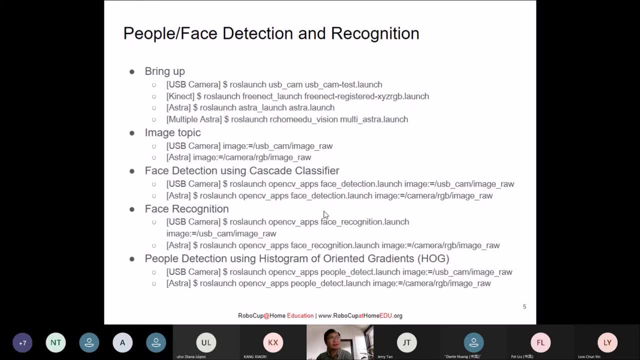 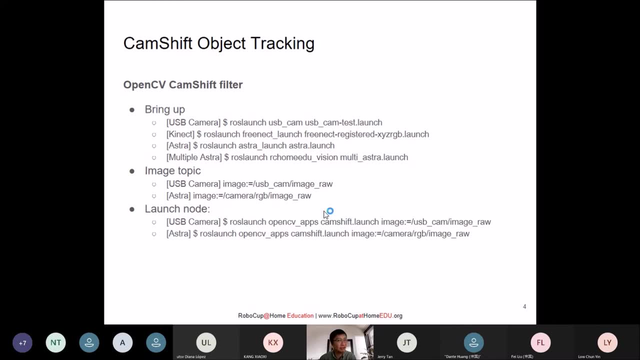 Right. so before that, I want to show you how to use the CAM shift and so on. Okay, so just now let me review a bit what you have just seen and also how you can use it for your development. So just now we show you, for example, this CAM shift example. 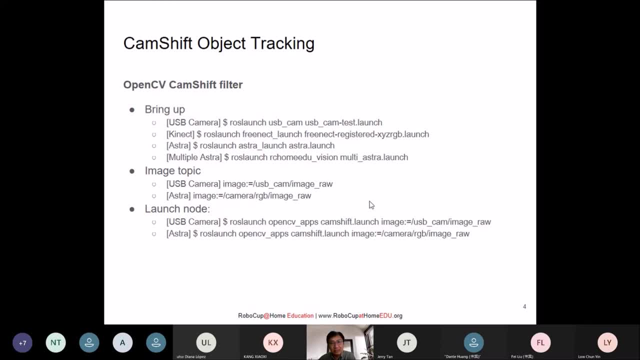 Then you can see we actually have a little bit of a demo. So just now we show you, for example, this CAM shift example. Then you can see we actually have a demo. Then you can see we actually have a demo. So you can see we actually input the image into this CAM shift algorithm in order to do the processing. 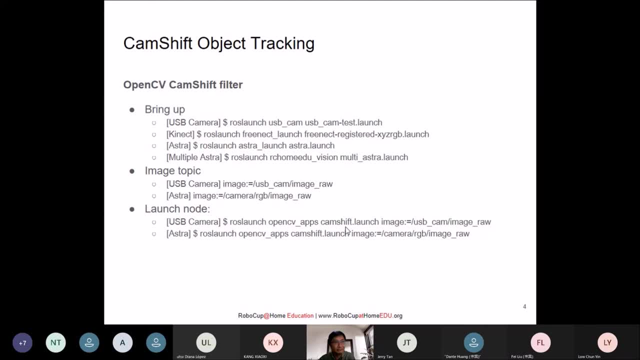 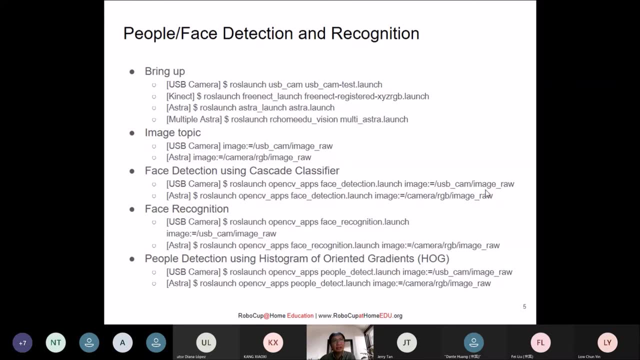 So you can see, we actually input the image into this CAM shift algorithm in order to do the processing. Okay then, if I'm not mistaken, just now David actually show you like how to find the image topic. Okay then, if I'm not mistaken, just now David actually show you, like how to find the image topic. 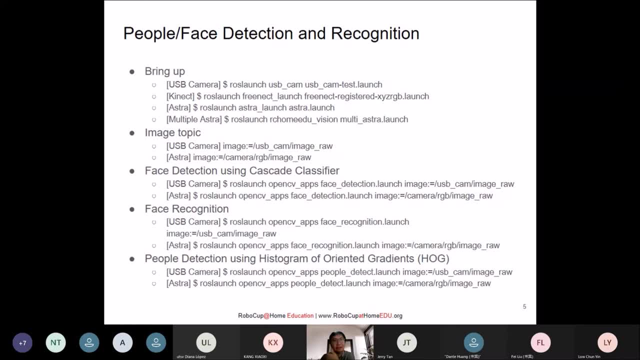 by using the ROS topic list right. So I hope by now you know what is the ROS topic list? It's actually to list down all the topic that currently active when you launch the application. It's actually to list down all the topic that currently active when you launch the application. 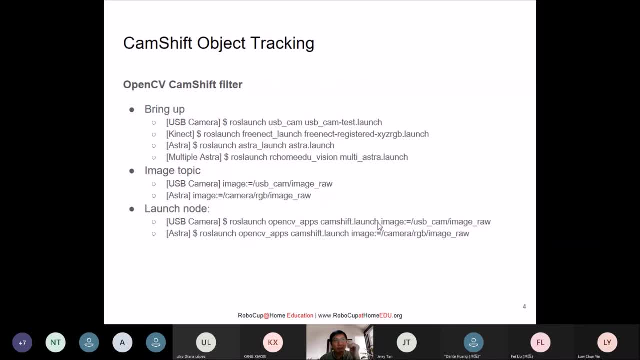 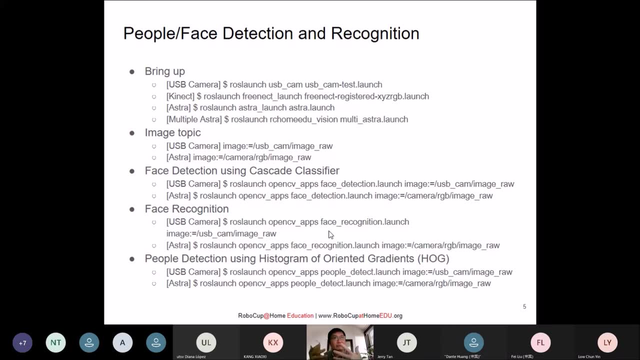 So, for example, when you launch whether the CAM shift or the face detection- So, for example, when you launch whether the CAM shift or the face detection and recognition or any of this, it actually will generate certain topic that will give you some. 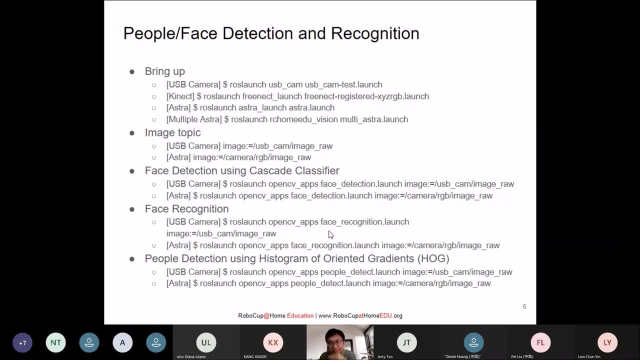 and recognition or any of this. it actually will generate certain topic that will give you some. for example, if you still remember last week, when we do the speech recognition, You use the KWS data or the LM data in order to get the result. 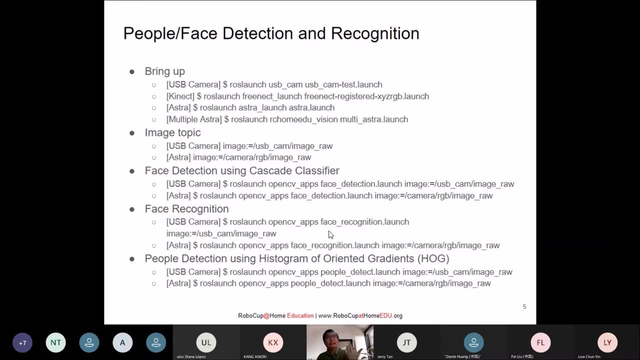 right. so similarly in today's example, for the cam shift and also the face detection, face recognition, they also actually output the result in some form in certain topic. okay, so the the way, how you want to know all this is like. of course, the first thing is like you can. 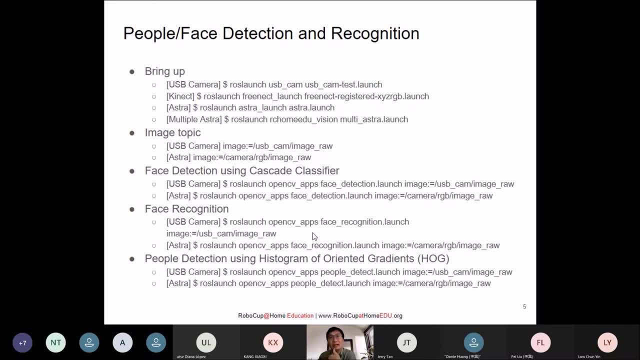 read the documentation of this in the wiki or you can open up the source code because, like these are all open source, you can actually open. open up the source code, which is just now david show you where. where are the source code that you can read, like what kind of topic that they actually publish? 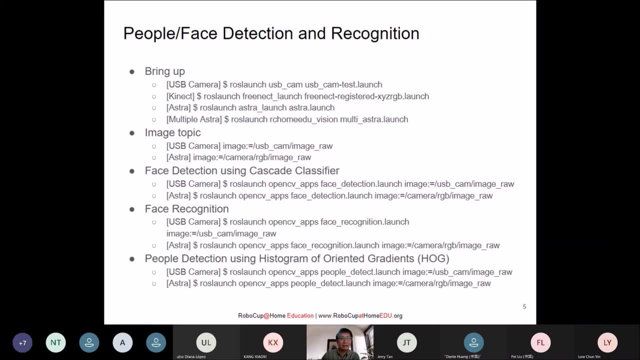 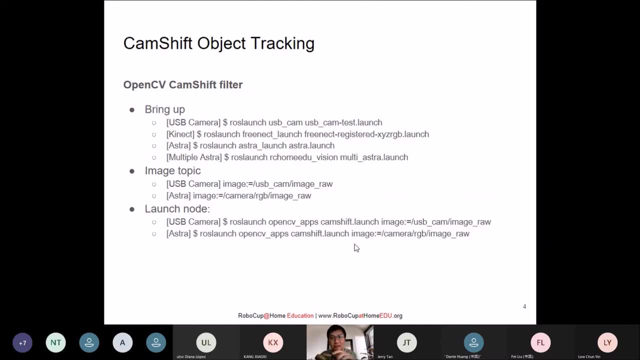 for certain result. but i remember, if i'm not mistaken, like if you run this cam shift you can find something what we call the result box or something rectangular that show you the result area and then inside there it actually have the x- y value. so by subscribe to that particular topic you can actually get the position of the detection. 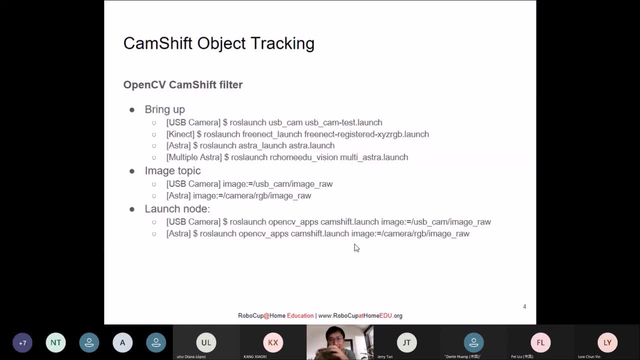 so when, when, in this chemistry example, when you detect certain thing, it will have a box. that box, that that uh- how to say it- will uh indicate the location of the things that it got detected. for example, like if you want to find something red or blue, just now you can see. so it actually. 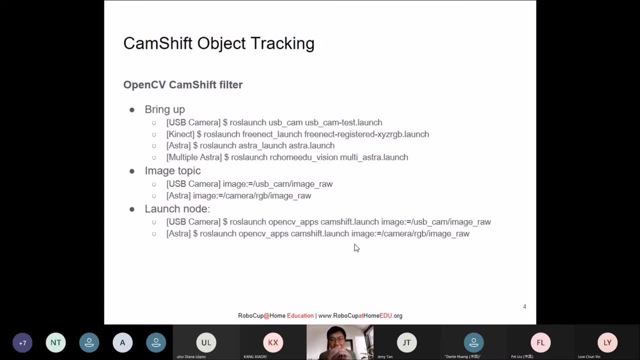 like um, have a box that enclose that area and then the middle of the box, the x, y value is something that being published out as a topic. okay, so you can find this information by read the um, uh, ross topic list and also to find uh from the uh source code. i mean, like this one is um last time. 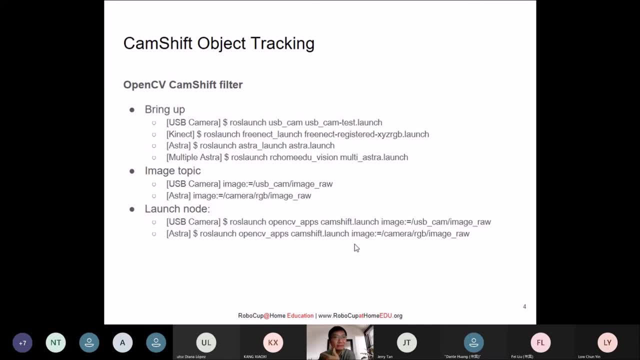 when i look at it, yeah, it is quite obvious that you can find all this result that you might want to. and who are you guys? it does notики. you can not just subscribe to this result, and then the next thing you can do is you can subscribe to the mentalafft that you might be able to use. so 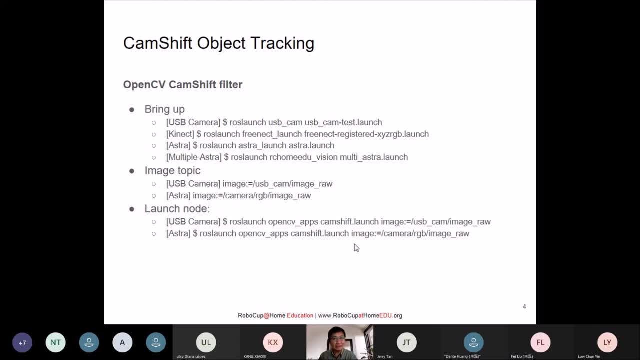 without changing any of the original source code. you can just subscribe to this result and you can use this result for some of your application. for example, a very simple application is like um. you can actually read out whether your object is on the left or on the right or on the top. 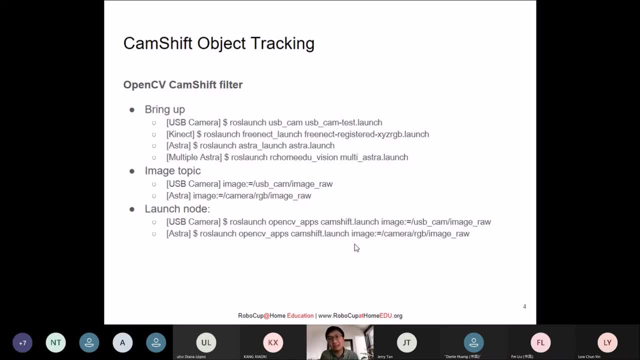 And also for the face detection and face recognition. I give you an example, for example, like if you make a robot service robot, for example, a receptionist, or a robot that man the counter in a hotel and so on. So when someone actually enters the view of the robot, which means it starts to detect certain faces, then the robot can start to greet the person. 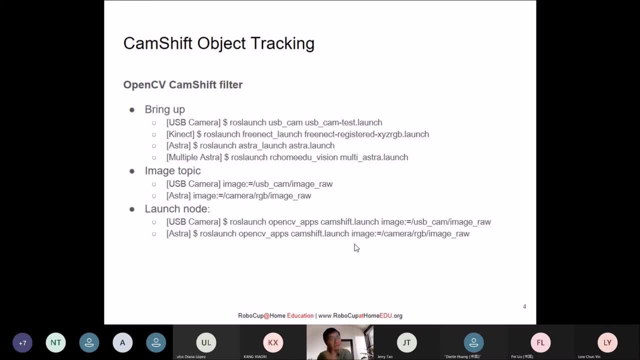 And if, let's say, you use some other tools, for example, you can detect this person is whether it's a male or female, then you can address the person appropriately. Then your robot will become more intelligent. So this is how you create an application from all these tools that are available for you. 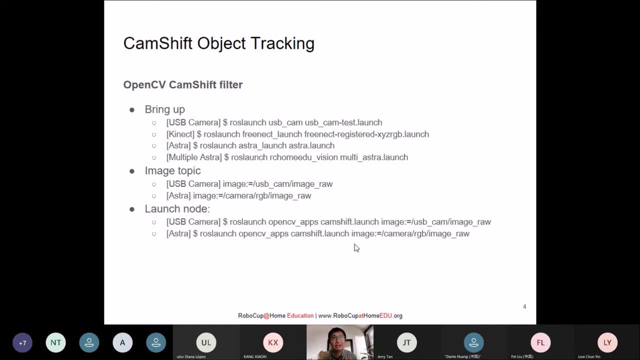 So this is one example that I can show you like you can detect a face, then you can give the greeting and so on, And you can use the recognition by every time. if the same person come to your robot, then your robot able to address the name. 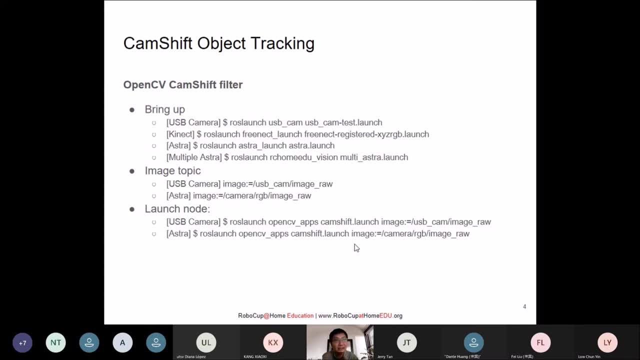 Because, like you can use your voice interaction to record down the name, like just now what David have done when recording the Max and so on. So you can actually do a lot of development by combining whatever that you have learned previously with the example here, so that you can create a lot more new application from here. 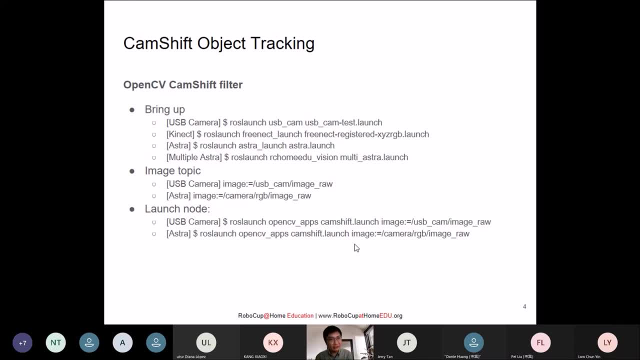 Okay, so this is just a few examples that I would like to share. Another point that just now, in the example that David showed you when it learned the face of the Max and then when another person come in, it also detects, But actually we don't realize or we don't really look into the value. 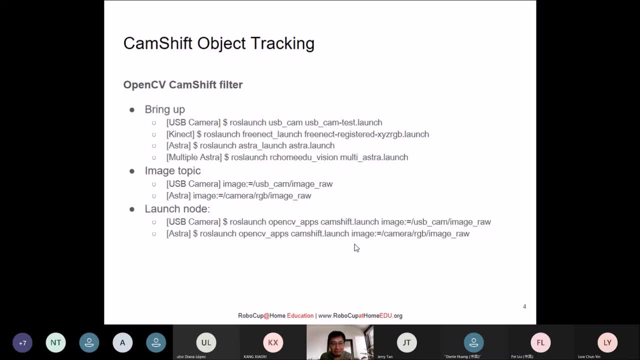 Okay because like the name Max, and behind it is actually the confidence level of the program to say like how much Okay This person look like Max. So there's a possibility that when it detect- so when it make a box of the face- it's actually just to detect the person. 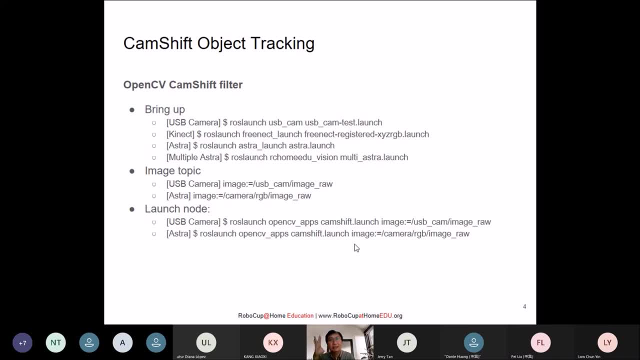 But for recognition you need to look at the confidence level. If the confidence level is too low, it only indicate that the program recognizes a face, but not sure whether it is a Max or not Max because, like, the confidence level can be too low. 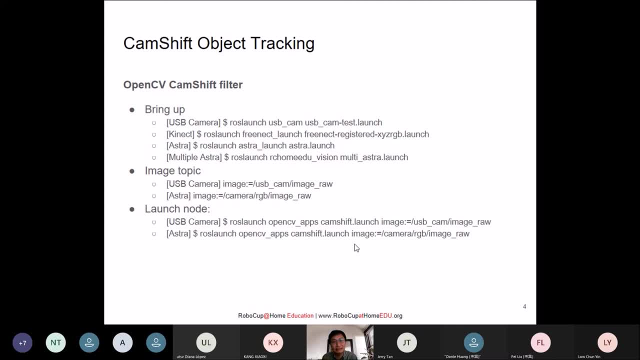 So if just now David tried to do the same thing to learn For another person and it might give you a better result. So that is my observation from the demo just now: that later on, if you want to use the face recognition, you might can try to learn more person in the scenario so that you can have better accuracy and also take note of the confidence level. 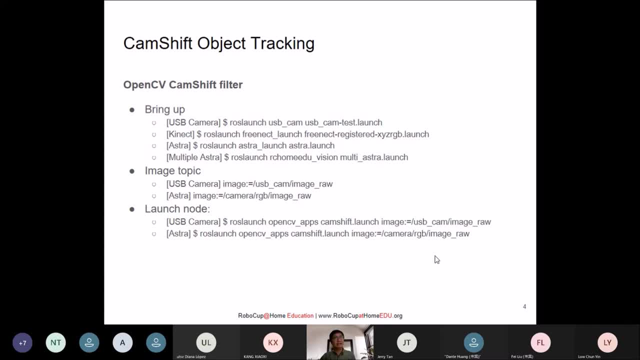 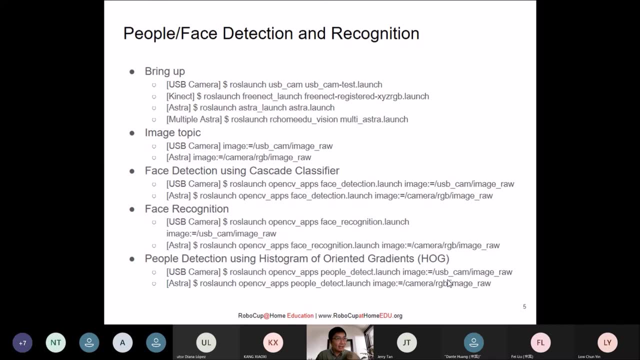 Okay, right, Okay. So that is my review for the demonstration just now And so far, all done, So far. all the examples show you is by using the camera color information, which is the RGB information, because, like for cam shift and face detection, we are using all the color information. 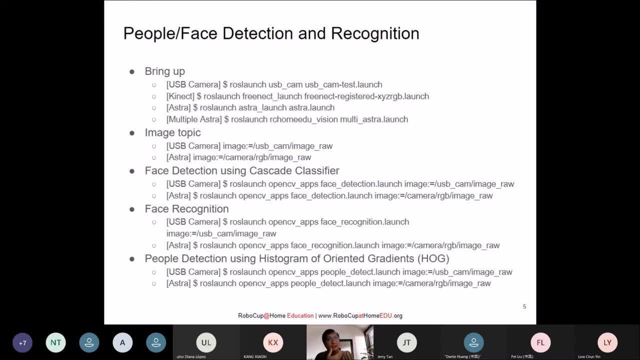 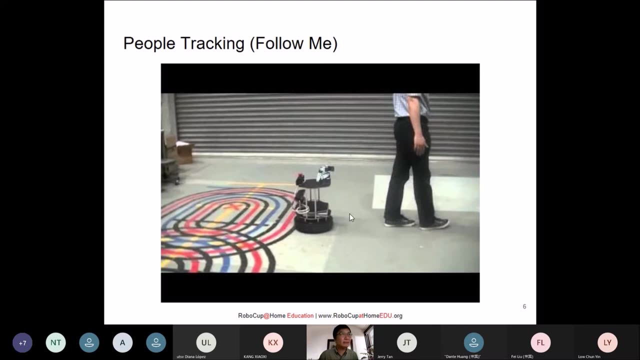 But what happened to the distant data or the depth data in our RGBD camera? So what we can do with that. So one of the example that we use a lot is for these people tracking. So I actually have one example here, but okay, later on we will show you the demo when I pass this demonstration to David to show you the demo. 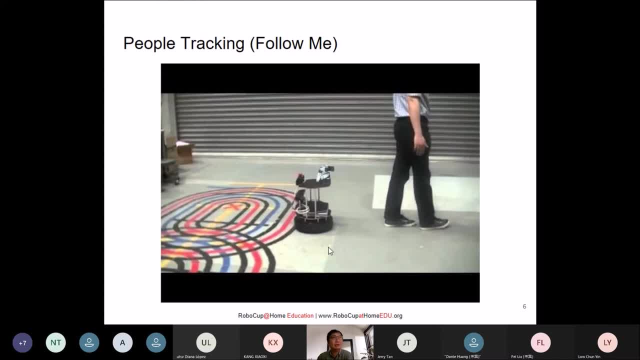 So you can imagine like we have this robot and it will move around, and then we have the RGB sensor behind here that actually track object in front. Okay, then it actually measure the distance, and all this will have the point cloud for us to do the calculation. 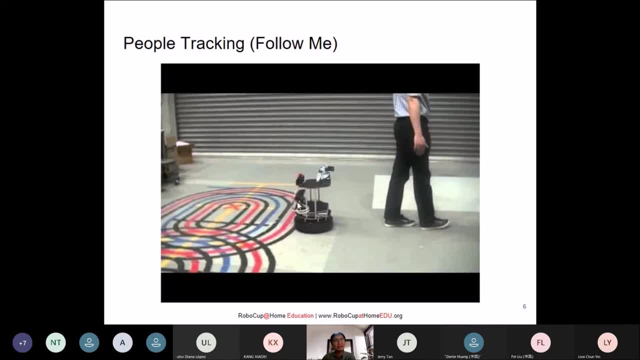 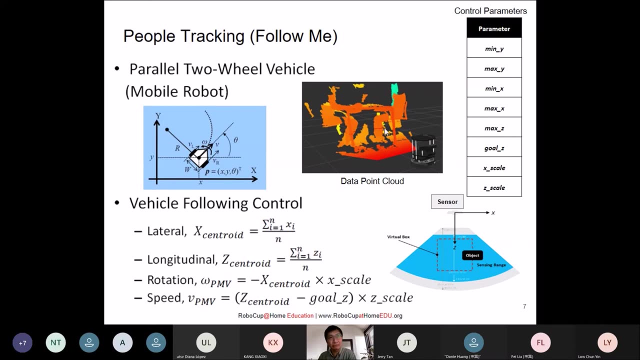 Okay, So try to imagine this. So try to imagine this scenario. and when this robot try to scan the environment in front, it actually get a lot of point cloud. Okay, so if we put this into this algorithm, so this is the point cloud that obtained by the robot. 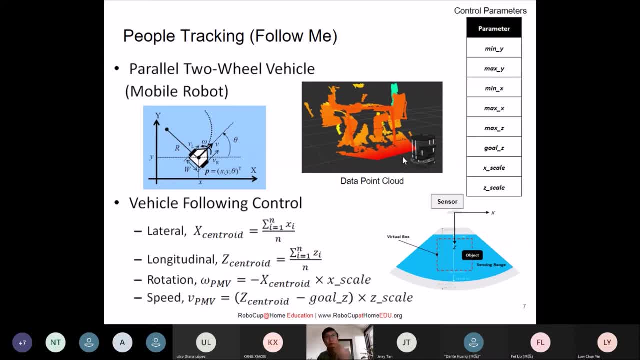 So we can see, like all this point and the color is actually red is nearer to the robot and maybe green is further from the robot, So we can see we actually able to get the distance. Okay, And all this point by try to imagine, if let's say, like this is a sensor which is the robot, and then the person is in front and we have the person inside what we call the virtual sensing area or sensing box. 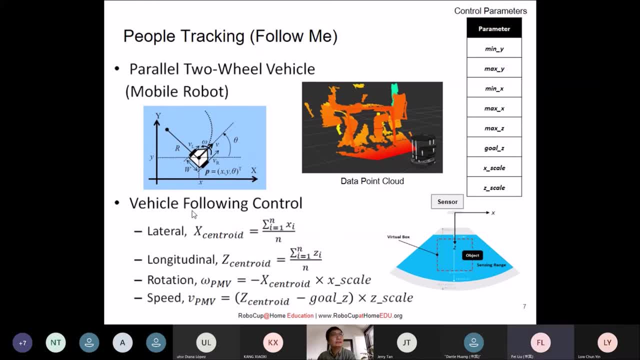 Okay, So what we do is like in this follow me program. it have a very simple algorithm that it try to calculate the centroid of the object in front of the robot. Okay, So it can be like: how many point at all this point? where is the center of that person? 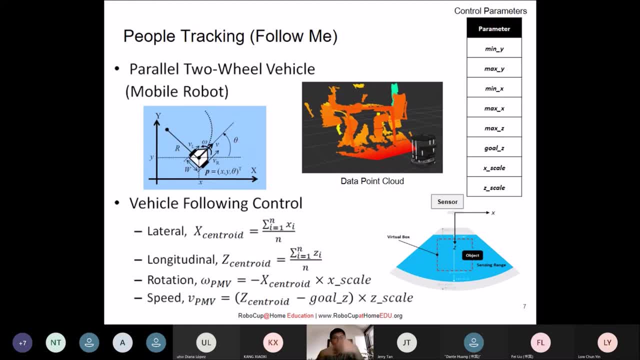 Okay, That person because, like when you have all the point, when you calculate, the center of all these point is actually the centroid of the object in front. So it using this centroid to track the position, whether in a lateral form or in a longitudinal form, in order to use normal, like p gate type. 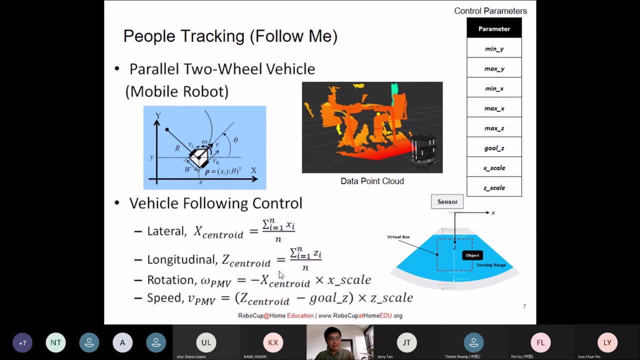 E value. So this is a PID, just a P gain, which is two times a certain X and Z scale. So X is in the lateral direction and Z scale is for the longitudinal direction. So it just times with the difference. So you can know like this control system is very simple. 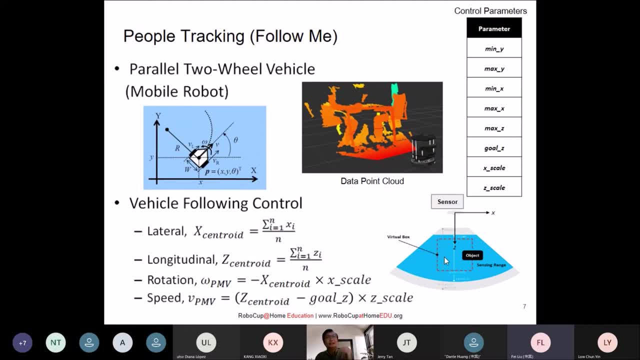 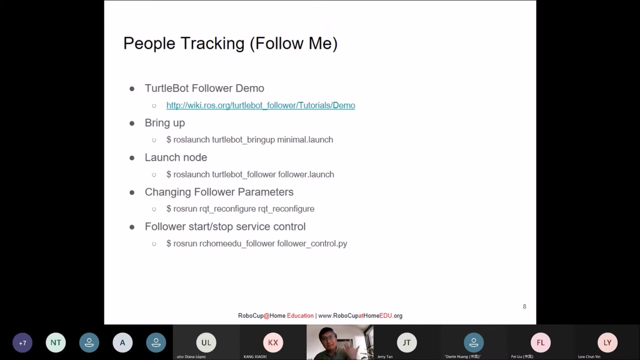 P control, So to find the rectifying behavior of the robot in order for the robot to track the person in front. So this is basically the simple algorithm, But if you want to know more, maybe you can read this thing and also the follower code after this. So with that in mind, 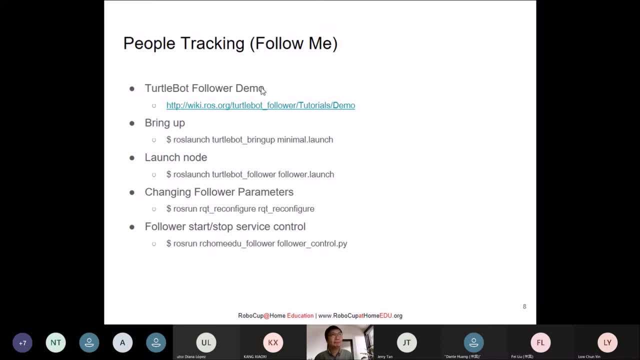 we can actually run this people tracking, which is we call it the follow me example, So you can find more information about this follower example over here, And in order to run this, we need to launch a few things. Okay, so this is where you need to install the TurtleBot package. 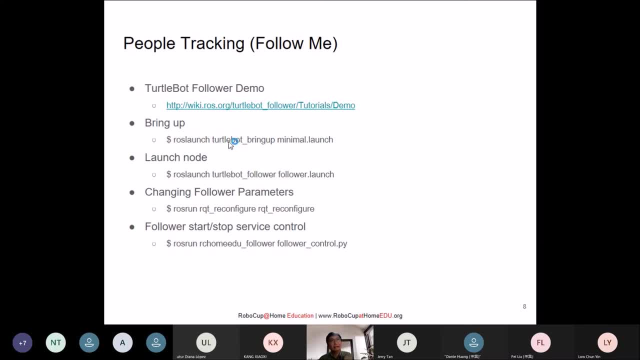 But of course you can implement this by your own. But it's easier if, let's say, you use the TurtleBot package because, like, this is part of the demo that come with the TurtleBot package. So we first, we launch the TurtleBot bring up, which is similar like our bring up in the sensor. 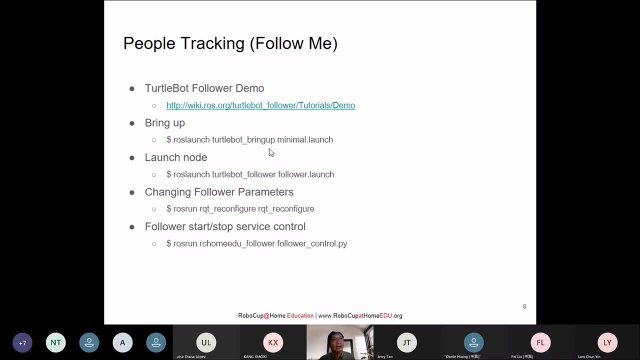 or the or the audio that it try to launch the function. So over here we use the minimum, Which is it make the TurtleBot in standby that it can actually react to our instruction. Then we launch the node which is inside this follower So we can see like inside there. 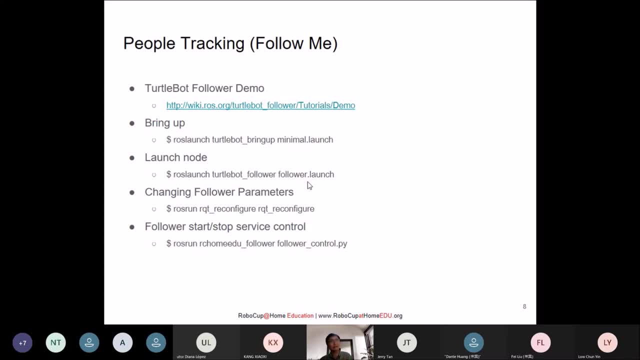 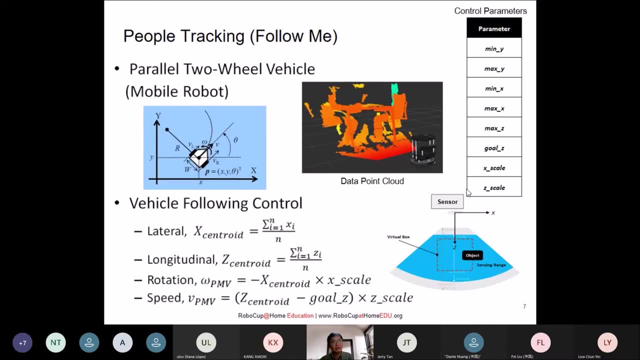 there's a package called TurtleBot follower under the third word package and got a follower launch And we can change this follower parameter And this parameter is: this is all this value. So how big? or you want to be small, very narrow or any different parameter of this box that will actually change the behavior or the sensitivity. 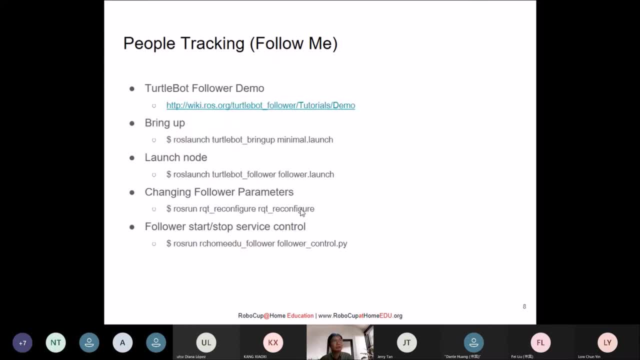 of the tracking. okay, so you can use this. um rqt reconfigure is something like slider to change the parameter. and also we add in one start stop control, which is a follower control in our um uh rc home repository example. this will be useful if, when later on you want to add this. 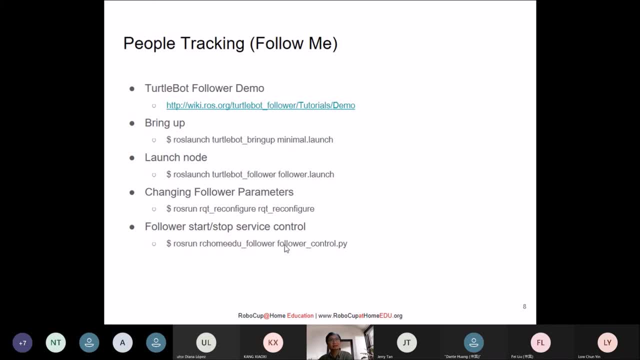 follower function into your application so you can use your python code uh in a programming way to actually start and stop the following uh behavior. okay, so this is the example that, um, i would like to explain here, but now i will pass the whole thing back to david to show you this follower and, if possible, david, please also show this reconfigure. 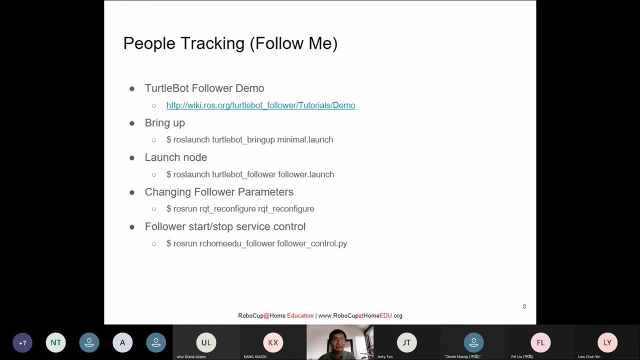 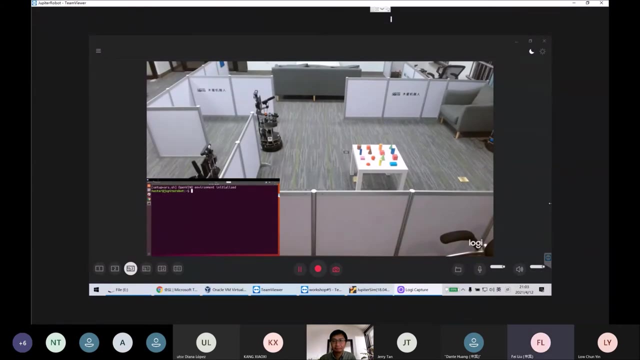 uh to see how to actually do some adjustment on the parameters. okay, david. okay, thank you, professor. now are you seeing my screen? oh, can you see the screen? i hope it's okay now, here is the office of uh computer robot and you can see several robots here and 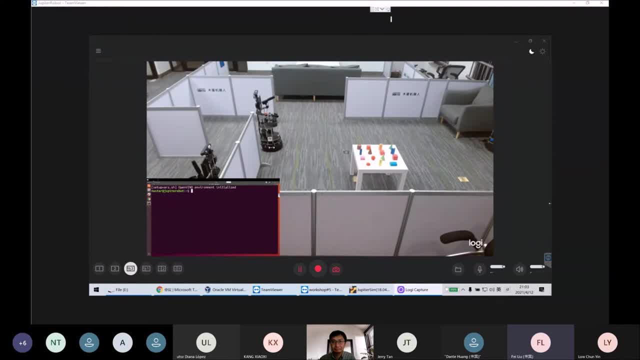 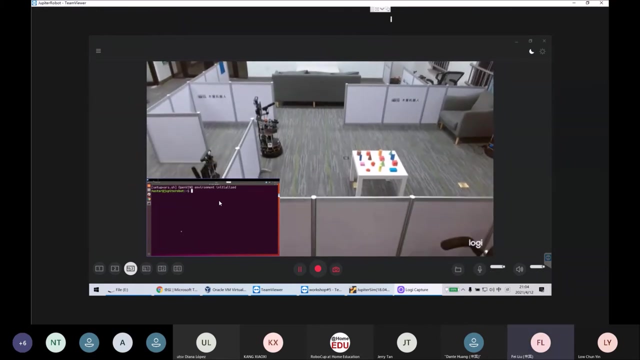 the robot, uh, stay, stand in front of the camera and uh, he is ready for the demo. so in this screen you can see the left button. there is a computer screen here, a little one, a small one, which means this is a. this is a program file of this uh robot. now i will start uh to show the followers, follow me demo. and the first: 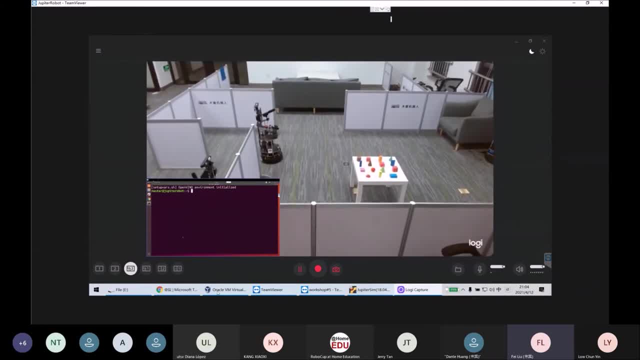 thing is we need to launch the pre-op robot for the computer robot. we have, uh, we have the our own. uh, bring up the launch film to be the robot, to bring up, to be the robot, bring up launch. so the robot is ready. i won't even 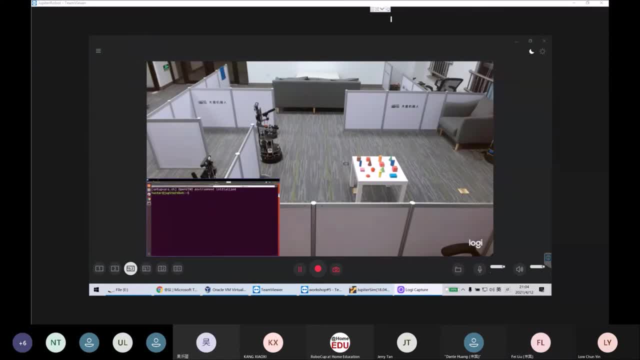 okay, and then the next is rose launch. uh, to try again and i'll teach you the gun. can rose launch asking home and you can see the robot is start, uh, start to follow the people in front of in front of it and people can and go around in the office. okay, very well. 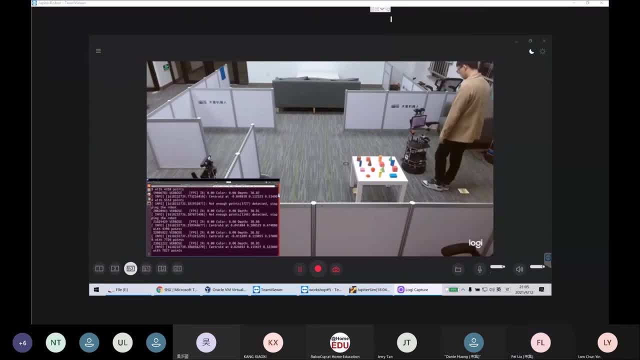 go back and follow. it's much better for the robot to follow the the people go. go forward, not go for back, backward. can you turn the robot to this side? can you turn the robot to this side? can you turn the robot to this side? 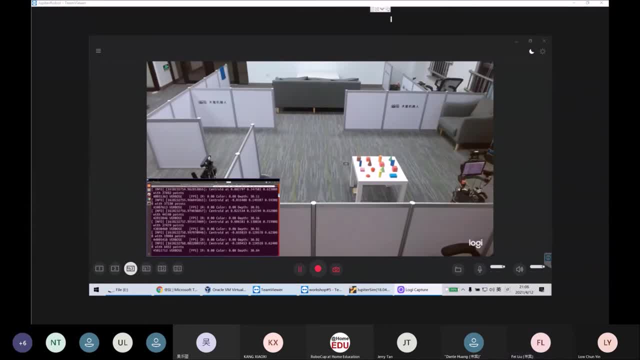 yes, yes, yes, the robot can recognize the, the wall in front of it, much better than the people in front of it. okay, okay, very well, say that, did you try? you can see the uh results of recognition. it shows you the result to uh, the, the follower program. 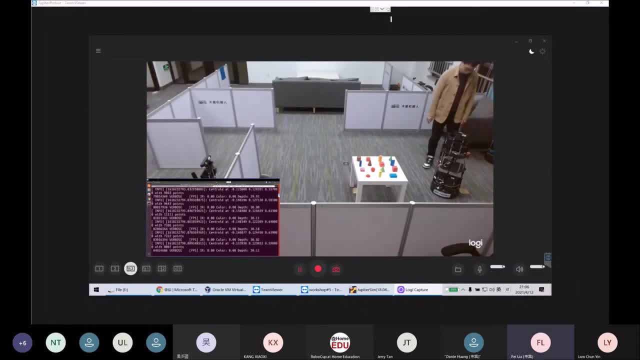 to show you the result of, uh, depth points. okay, very well, uh, professor jeffrey, uh, do we need to show the follow-up command? yes, your initial right. okay, there is also a command here. uh, i mean a node, we can use the command to control the follow-up. 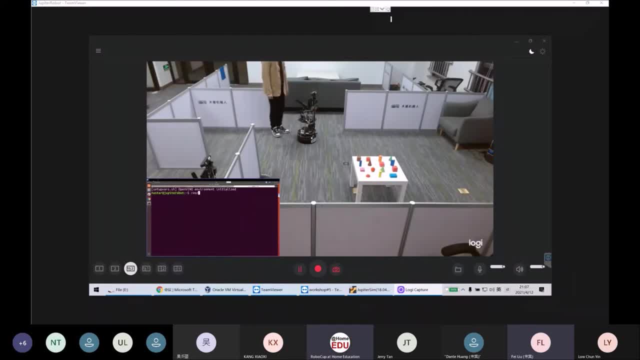 uh moment, which means rows. run uh control, stop p1. so there is this three command here and now i will use stop, the robot will stop. follow, okay, and if you want to start again, i can use f, the startup again stop, stop, yeah. if i want to uh shut down this one, i can use the x. 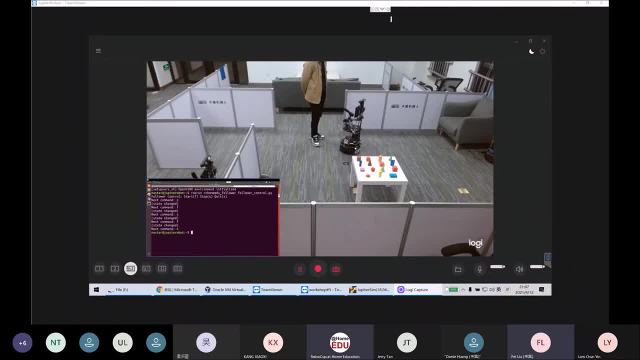 to stop this command under the robot view. start follow again, because the commander control is uh, shut down, shut it down. okay, jeffrey, this is uh demo for the follower. okay, you can continue the. you can continue with the euro example. okay, uh, now i will shut down the. 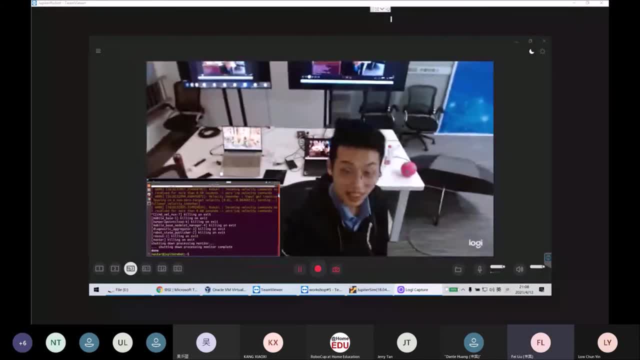 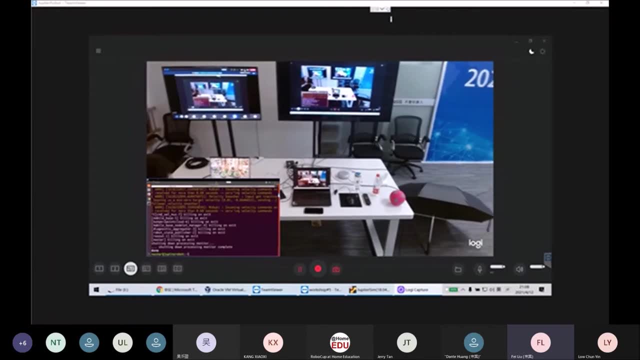 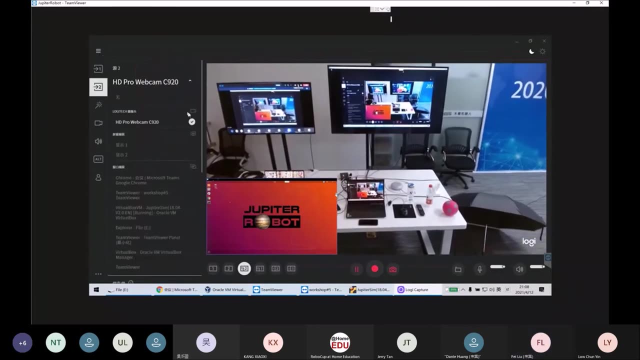 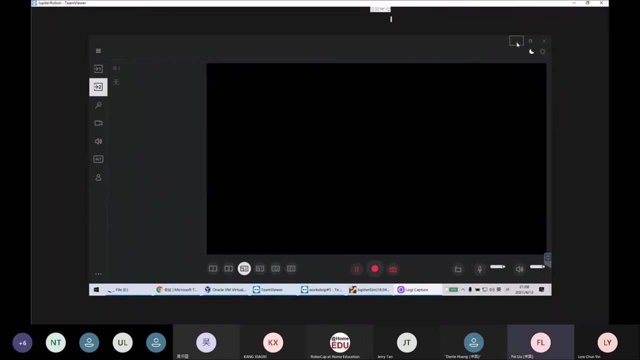 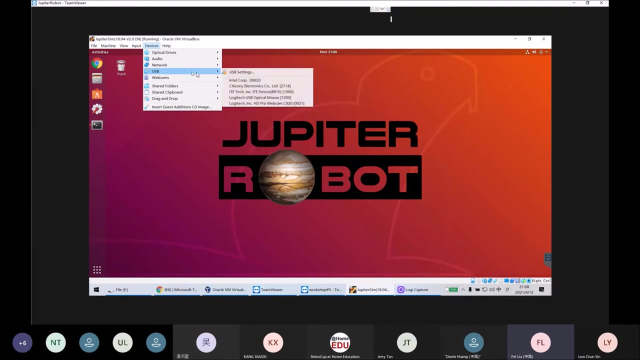 so for the euro, i will use another, another. i will use the virtual machine for the euro. okay, and i will. now i will go back to the waterboxd machine and i will input a device connect with this logic. okay, for the euro, and we have already set up the environment of uh open window in the uh. 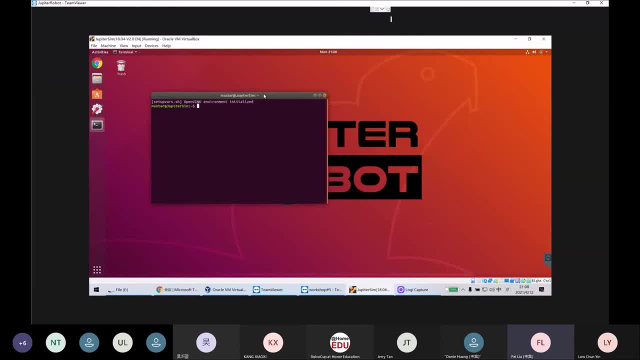 the jupiter robot. uh, jupiter robot, uh, jupiter robot, uh, virtual box, virtual machine. you can see here, well, open window environment is in naturalized, which means the open window environment is okay for this application, and we have several applications for this open window, the most important one. for the first one is the euro. 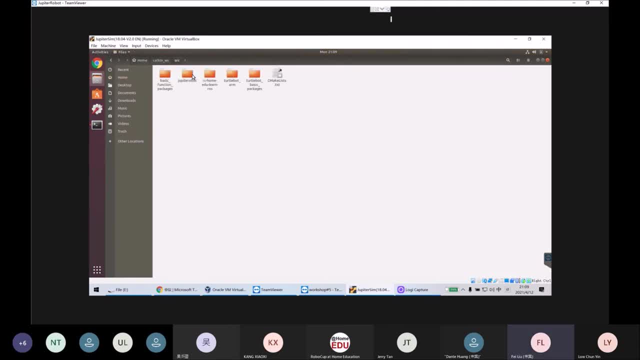 we have a setup package here: jupiter robot, jupiter robot models, open robot vision. robot vision open window and uh not here. we have uh yolo here and before we use the robot vision we need to configure the uh topic, which topic we will use for the vision. so we have 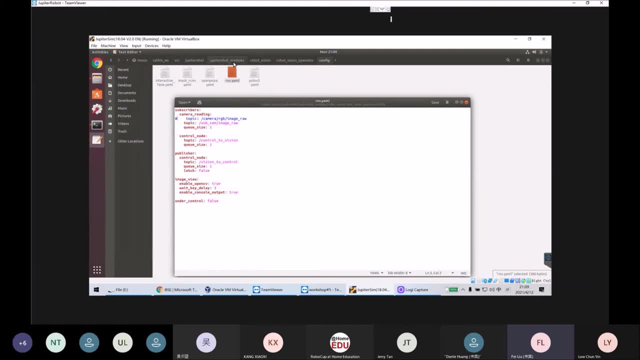 a config file. here we can follow the photo name to config one config photo and, uh, change the yours point one aml file to a target image. now we have already change the topic to the usb image and if you use the real robot, maybe you, you can use the camera, rgb imager or camera. 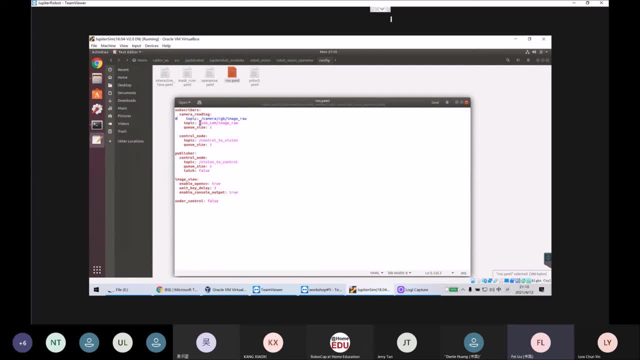 top rgb image으로. you can also change the topic name to your uh, to your own camera, for example for the astra camera or the connector camera. you can. you need to make sure that you use the rows Ну. figure out the imageick in页. write a topic name. Now I will show you the result. First we 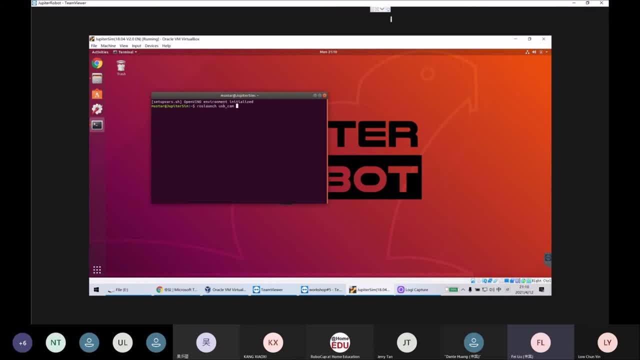 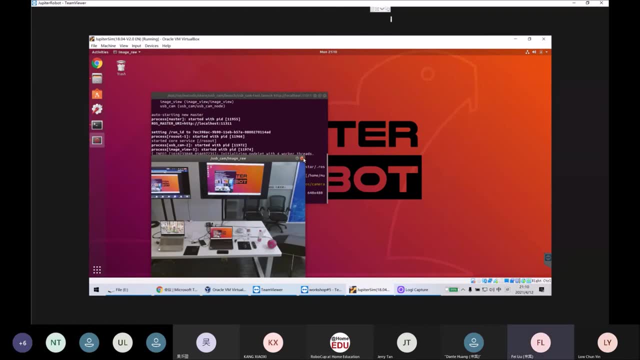 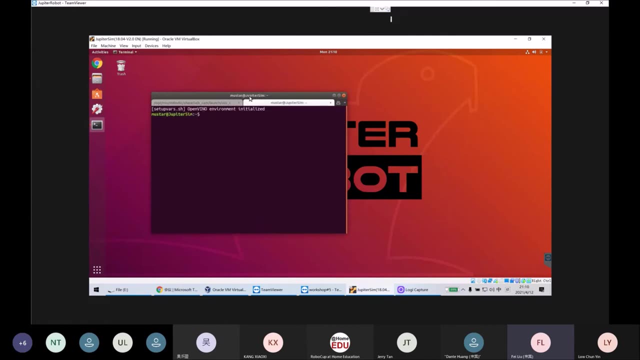 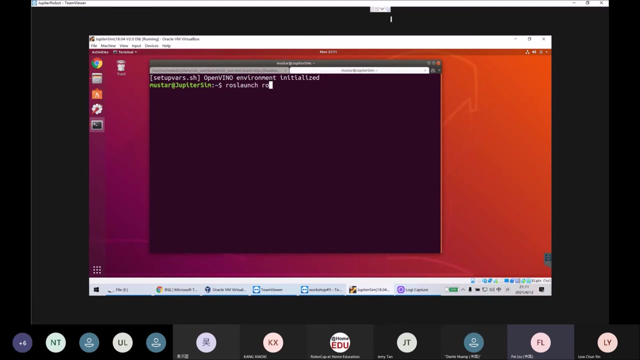 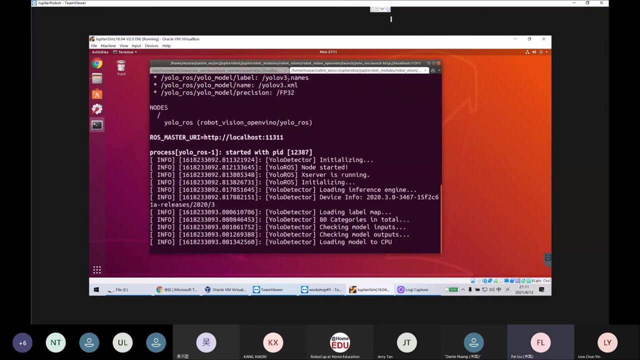 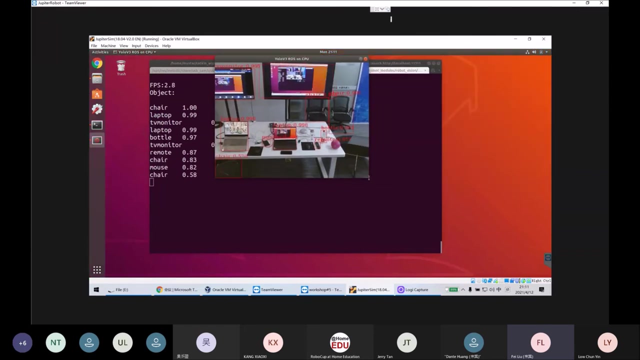 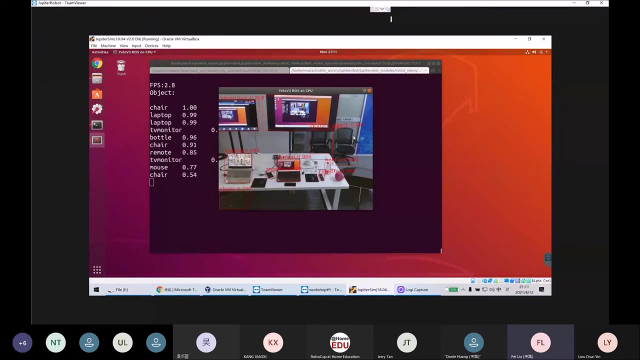 need to bring up the USB camera. Okay, we can close here this window and new tab: Open window- YOLOlaunch, We will start another window to show you the result of the open window. here You can see the program can recognize the different type of object in the image. 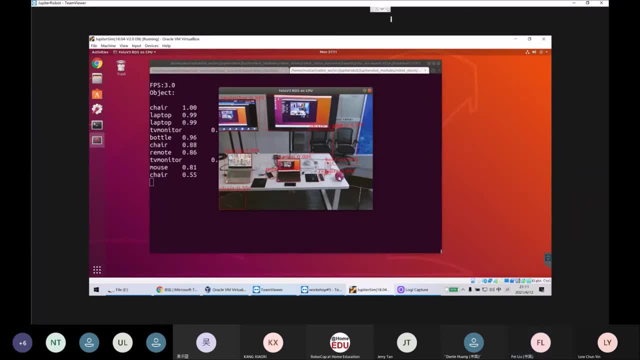 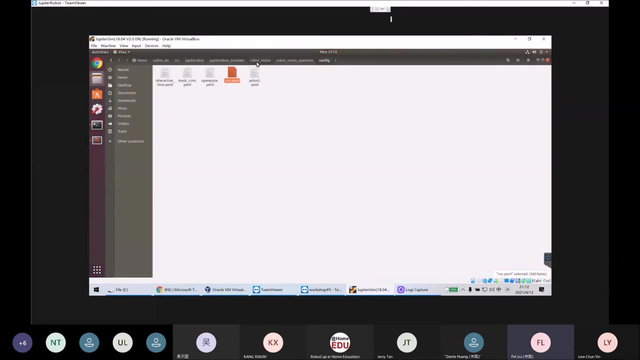 Here is the laptop, The bottle here Chair laptop. This is a TV monitor here. So the YOLO3 can recognize for 80 objects for the trained model. We can see the object name here: Models YOLO3, YOLO3 name. 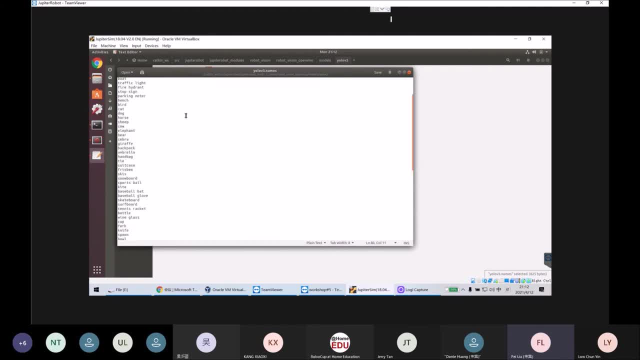 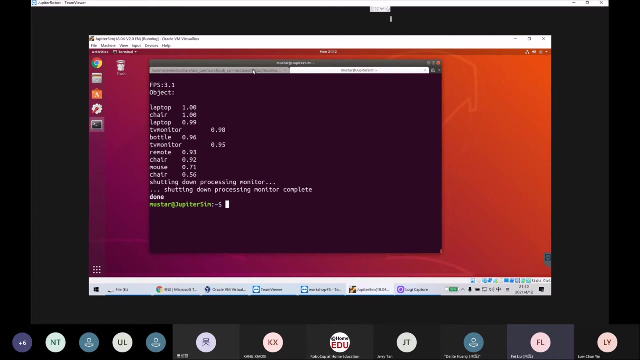 This is a list List for the recognized results of YOLO3 and the number is the 80,: 80 objects here, which means the robot, the YOLO3, can recognize Okay. another application is the open pose. I will show you the result of open pose to recognize the pose of the person. 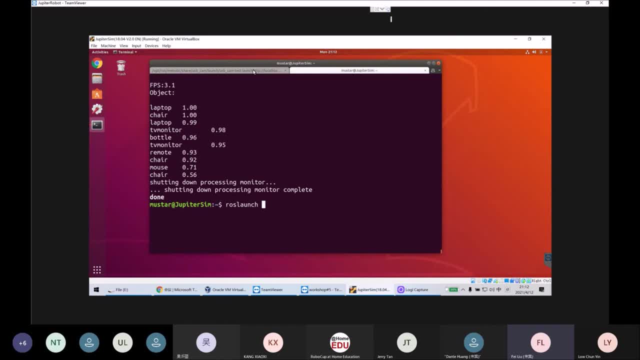 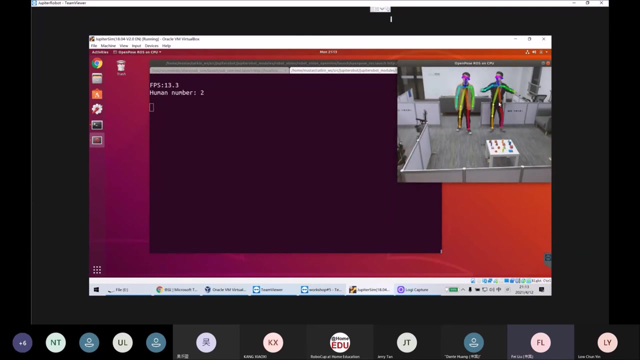 And the result and the launch file: Rose launch robot Vision Open window. Open pose. Don't launch, Okay, Well, I'll show it to you. I'll call it. Uh, okay, Hey, thank you. This is the result of the open pose to show you the post of the person recognized by the program. 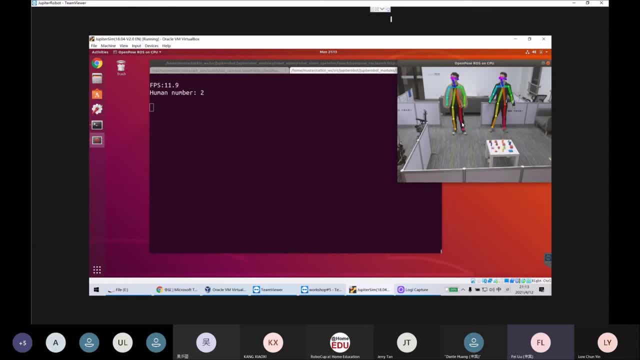 So you can see the different. different color means the different part of the of the people. For example, for the left Right hand- I mean it's my right hand- is a light, light blue And this one is a red. left hand is red, light green. 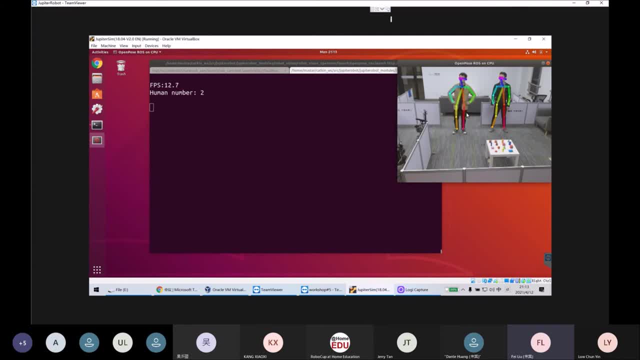 And this one is for the left, left left leg, And this one is for the right leg, And there is also the face detection result on the face of the person. You need to know, Okay, So we're going to need to know. 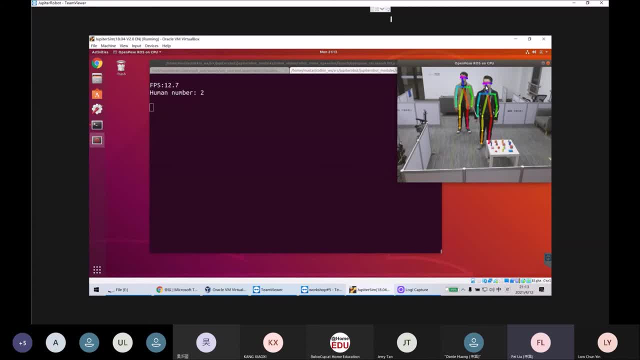 Okay, Can you go then Hold on again, Should we do it? You can see this is also the result of the eyes, The years and also the The center of the face. Okay, this is the result of the open pose. 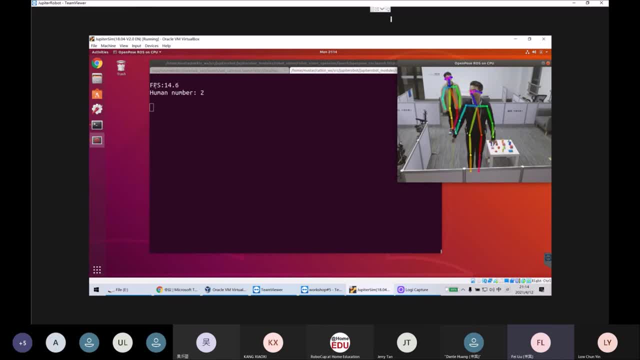 The real time. This is the FPS means the frame of per seconds. frame per seconds, frames per second for the processing speed. Okay, And we have also a, A demo for the interaction and interactive face. Okay, Well, let me, We don't. 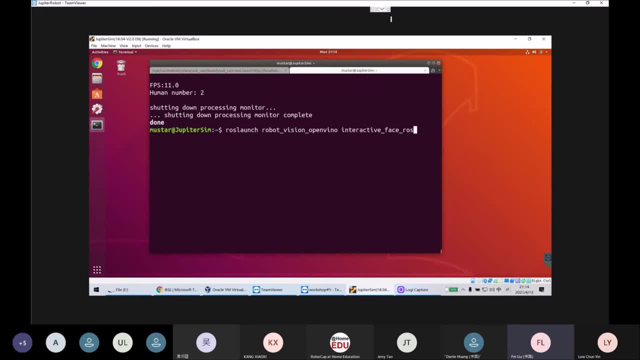 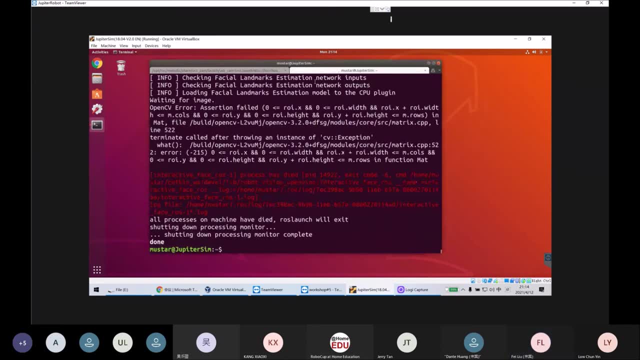 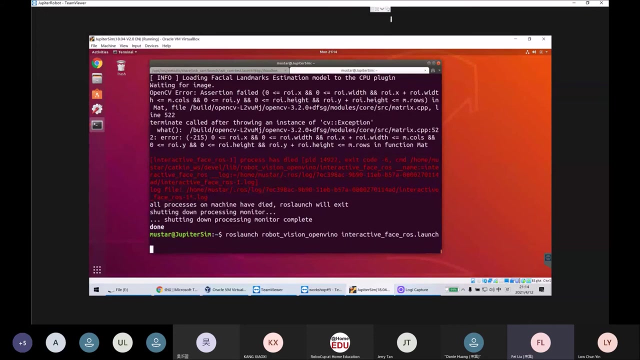 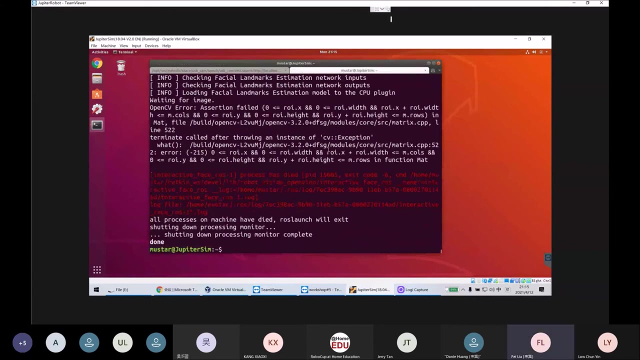 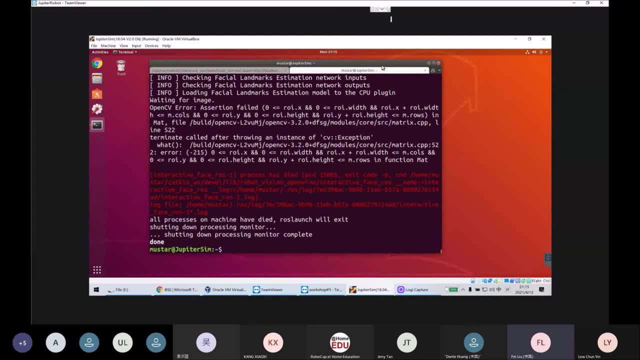 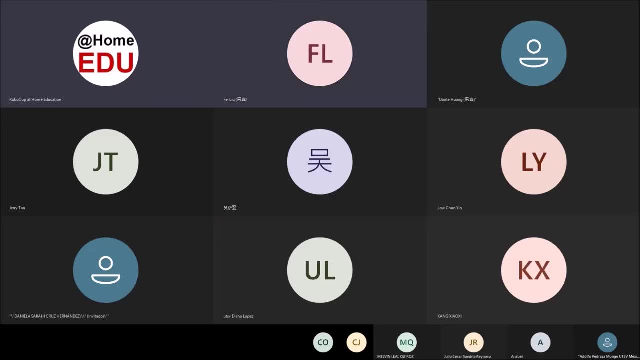 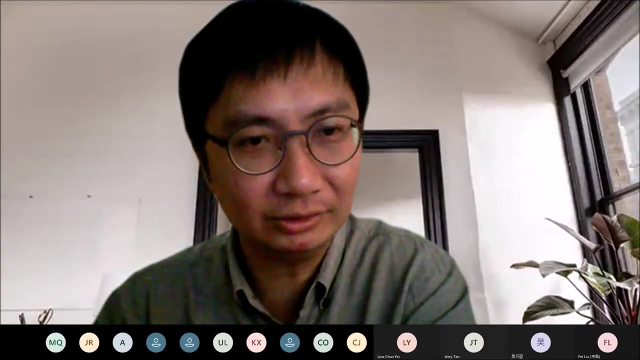 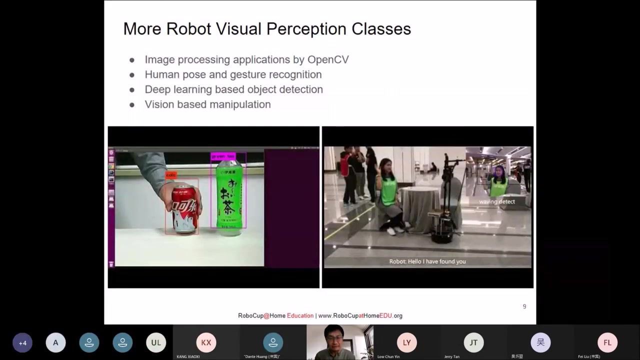 citing for this demo. Okay, that's all, Jeffrey. that's all, Jeffrey. Okay, thank you. So just give me some time because, like, my laptop is quite heavy, Okay, so let's back to Okay, right? So thanks a lot for the very interesting demo, And actually so just now. 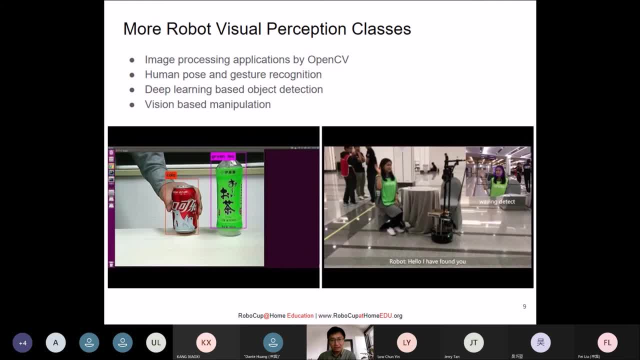 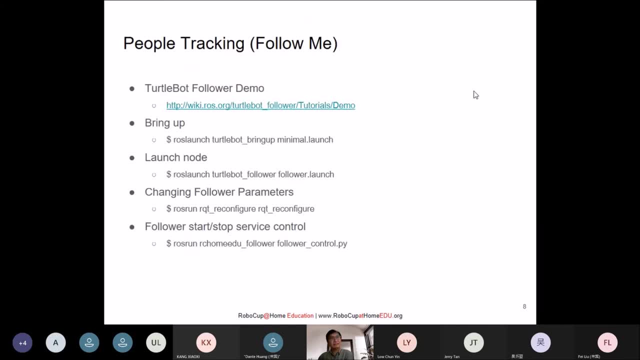 what you see. Okay, so I hope I'm back. So just now a few things that I want to review. So first, it's like for the follower. So the follower is a very useful application that you can include in a lot of or many of your service- robot development, For example. like in our repository we actually 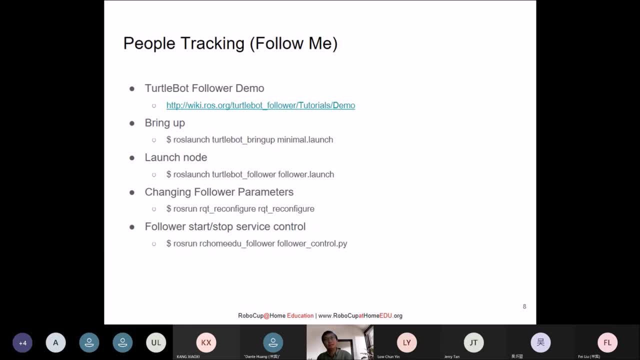 show what we call a party bot example, that you have a robot that can follow someone- Okay, and then you can take photos. you can do some interaction, for example, like speech interaction, answer some question, do self introduction and also tell jokes. do some performance. 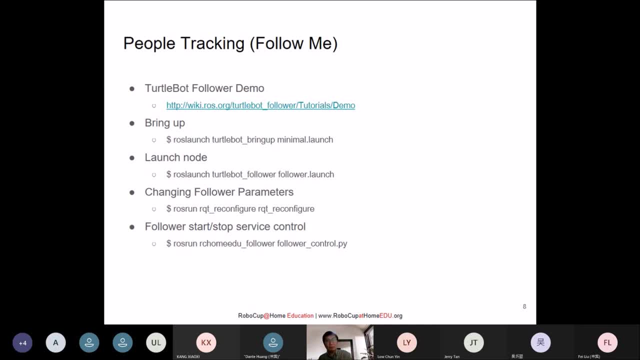 like do some dancing, play some song and so on. So with whatever that you have learned, like in the second week and also this today, plus the follower, you can actually make your robot very interactive. Okay, so this follower also, like we prepared the follow control, which is the on and. 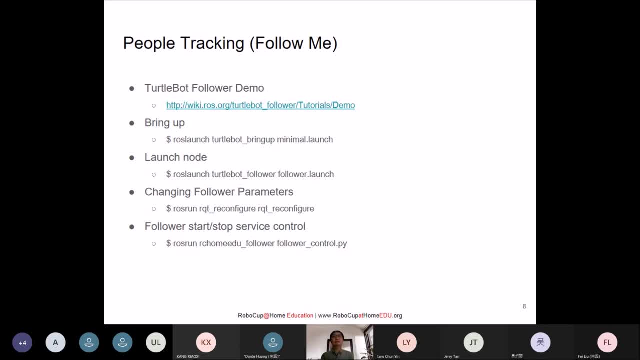 off button is actually to let you. Okay. so the follow control, which is the on and off button, is actually to let you able to like, for example, ask the robot to follow you or ask the robot not to follow you, so that the robot can stop over there. 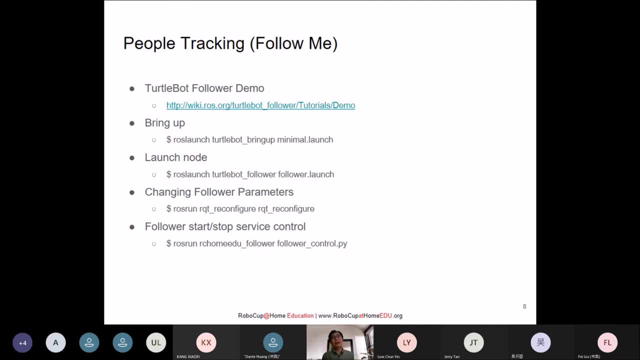 So a lot of interaction you can do once you combine whatever that you have learned in last week for the speech interaction with whatever that you learned today and also after this, Okay. so I hope, like you can be more creative, to see how you can input all these things together to come up with interesting application, of course. 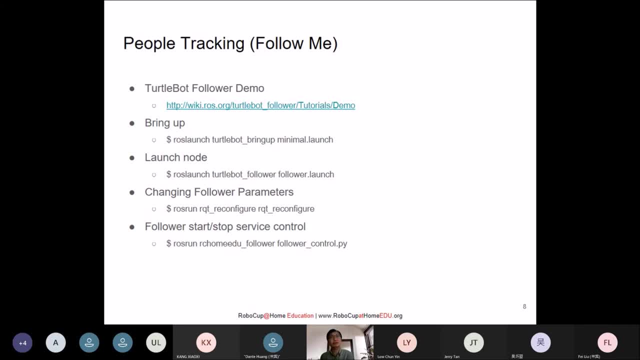 But, of course, if you don't have the robot or don't have something that can move, you can also use the simulation, But maybe we will introduce some later on to tell you more about how you can use the simulation model that available in the virtual machine as well. Okay, so this is for the people. 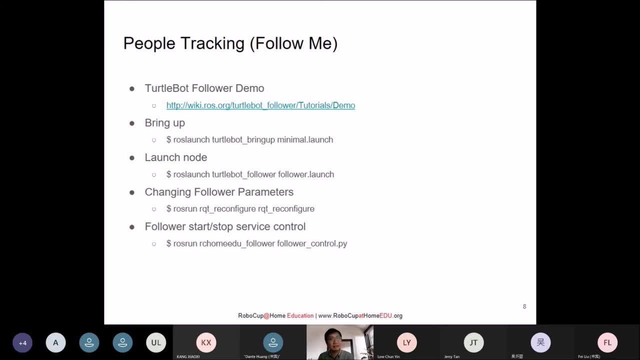 tracking. And one more note that I would like to explain, like because just now we show you the actual demo, you don't really see the data for the Hoi Cloud. Okay, we actually have a way to show point cloud and so on, but it's a bit too complicated um to show like remotely currently and and i mean 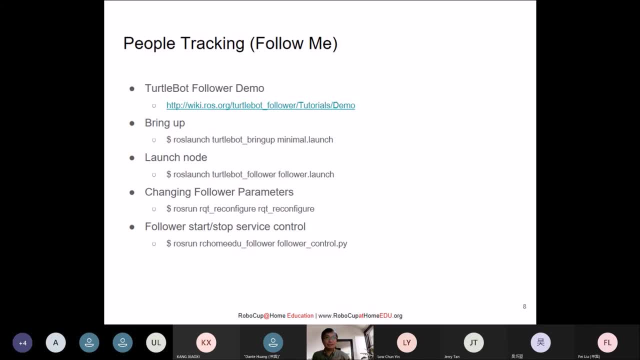 the, the robot, and also remotely on your left, that desktop, so you can actually, uh, try to see the, the, how to say the point, cloud data, uh, if, let's say, you have a like lgbt sensor with you, okay, because, like just now, i will show you in the first uh demonstration, i show you like i use the hand to. 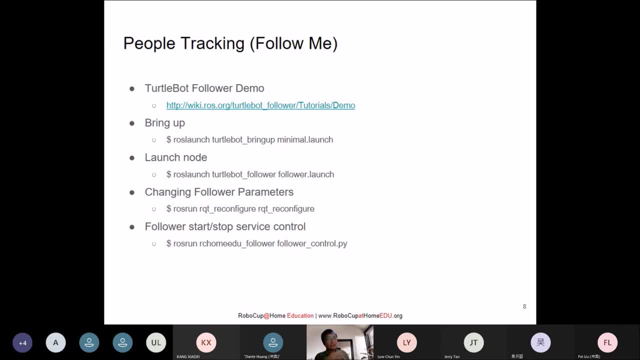 actually block the sensor and you can see, like, uh, we have the color, the black color, but we can actually show that in three dimension. okay, which is the rvs. okay, but maybe we will show you, uh, the next time when we have, uh, the setting, uh, to show you how it looks like in 3d. okay, right, but anyway, 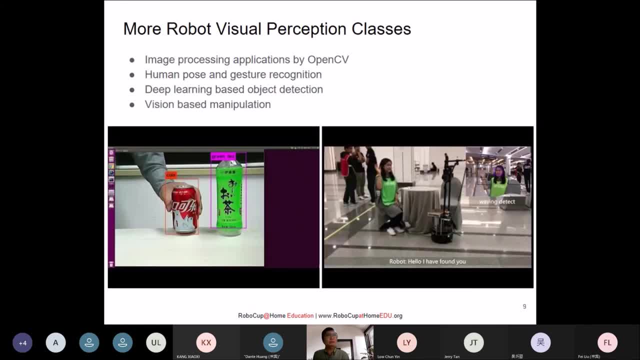 so let me proceed with, uh the content today. so, um, today we show you a lot of um interesting um uh application, uh that use the image processing, uh with the environment that you have. okay, even with just a simple camera you can do a lot, and even just now, before we stop for the follower, 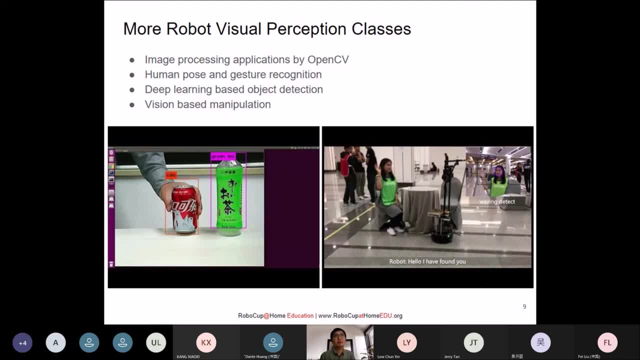 uh, i also like uh let um david to show you uh some deep learning based um object detection, for example, the euro tree and also the open vino. uh, on open vino, which is uh open post, uh, that you can do a lot of um very accurate recognition with the image, with the vision. okay. so, for example, like, 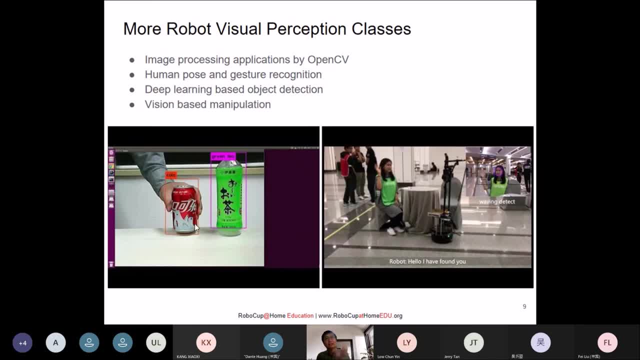 the yellow tree. okay, so this is the yolo example. you can real time recognize different object, okay. and also you can use the open pose to to detect the motion of the person right, uh, like what, like waving, and what that person is currently doing. so, with that you can have a lot of information. 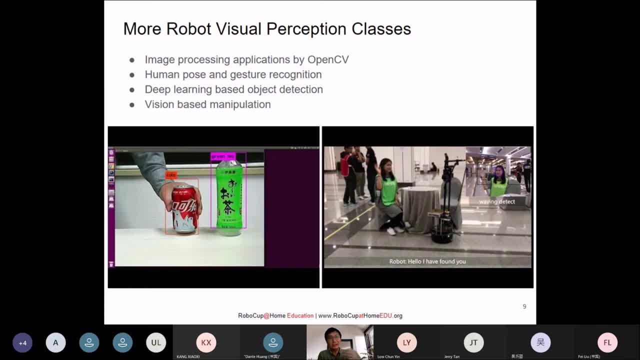 uh, for the robot to understand what happened to the surrounding weather, what happened to the surrounding in terms of, like, the user that the robot interact with or the object that the user interact with. so a lot, a lot of things that you can do, so like over here: image processing. 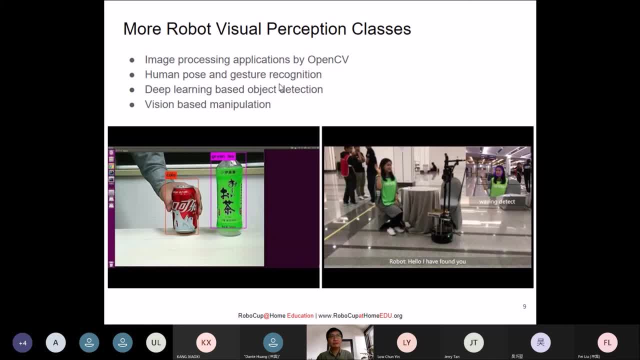 application by opencv, then human pose, gesture recognition, deep learning based object detection. so you already see, like many examples, and also these are all the framework already built in your virtual machine that you can explore because, like we only have like two hours today, it's not possible to tell everything in detail, but at 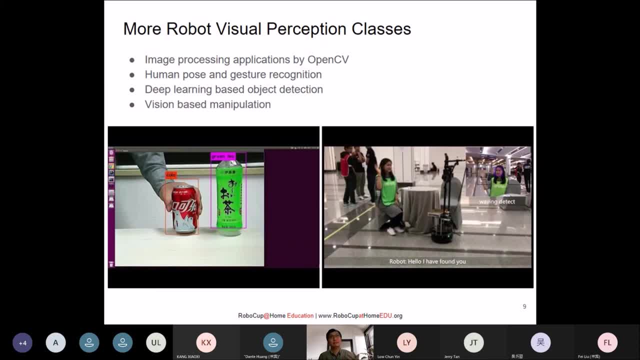 least i hope now you you know that you know like you have some exposed to all this information so that later on you can look more detail. but of course, if you want more information about certain part of the demonstration today, feel free to contact us and i will provide you more. 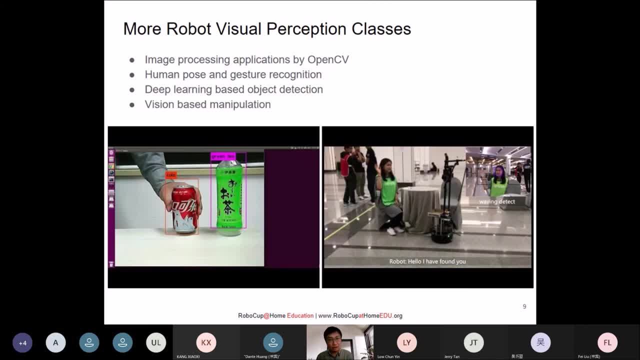 information, but everything that i show you today is already like open source. you can find the original source code in the virtual machine, so everything you can actually like look through, uh, inside the virtual machine, okay, and of course, like a vision based manipulation script. so this one is something that you add, the vision with the um that we will. 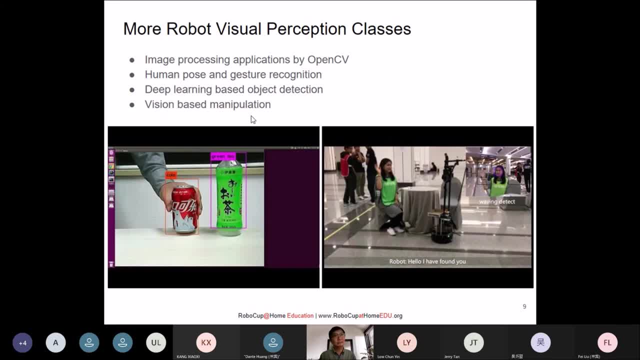 discuss, uh, when we, when we have the class for the manipulation. okay, so with that, um, basically, we have covered the content for today. uh, and i would like to discuss a bit, before we end, about the assignment. okay, so the assignment is to how to say, to summarize the things that you have learned and to see what you can do with the things. 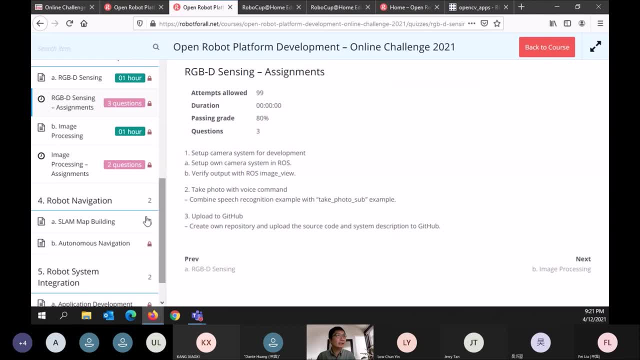 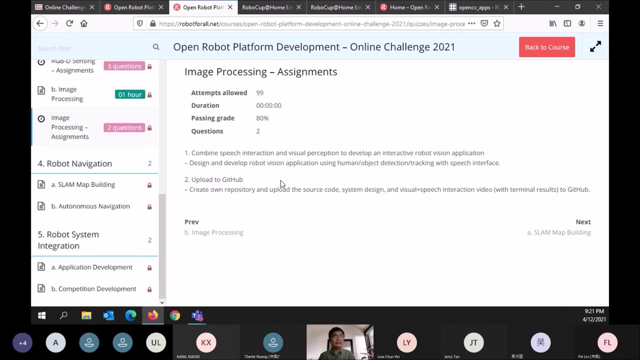 that you have learned. okay, right, so for today, the second assignment. uh, okay, the second assignment is this one image processing assignment. okay for this. uh, i hope by now, just now, i'll really give you like a lot of example. you can combine the speech interaction which is last week speech interaction. 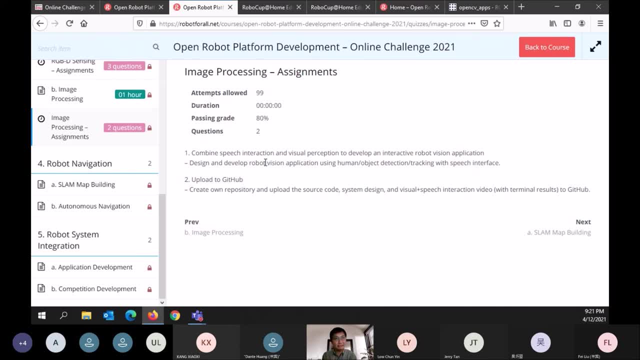 with speech synthesis and also speech recognition, so your robot able to say something and understand what the user say to him. okay, then you combine with the visual perception that today we have, for example, the cam shift example you can use, or the face detection that you can use. 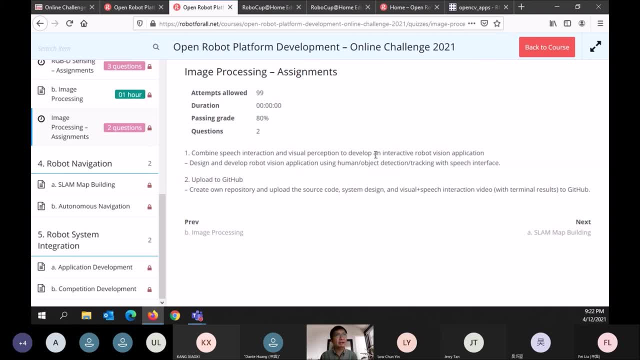 uh, okay, i will give you example after i read out this. to develop an interactive robot vision application: okay, so you need to design, develop the robot visual application using human or object detection tracking with speech interface. so i'll give you example very easy. so, for example, you want to develop a, a reception robot, receptionist robot- okay, for example, 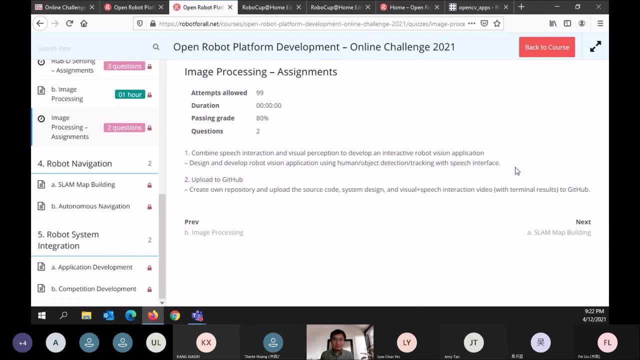 so all you need is just your laptop with the virtual machine and also just a camera. okay, you don't need anything else, you just need this, and this setting can be done easily with just your laptop. so once you have these things set up, so you just need to study how, for example, the face. 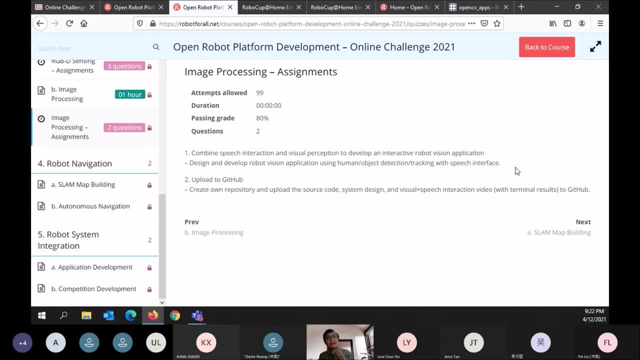 detection example. okay, so the face detection example will give you information about, like if someone actually within the the sensing of the camera, so which means like anyone that moves into the range of the sensor, then you can detect someone is actually appear. so for a reception robot. so when someone come near to the counter, what the reception robot should do should for. 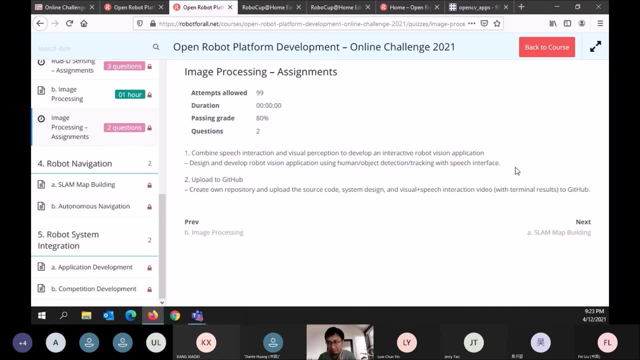 example, is to do a quick reading. okay, so, like, other than this reading, you can do any, uh, something extra. for example, like ask for the name- and this is where your speech interaction. but come in so you can ask, like what is your name? then you try to remember the name, or maybe, like it's within: 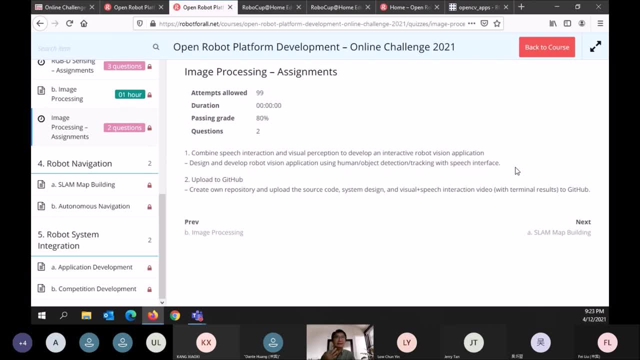 your database and so on, so you can do all this thing. behind there is just the logic that how you want to put things together, okay, and even you can go up to the extent that you can try to memorize the person, the name, so store in your database. we show you the face recognition today, then the next time the 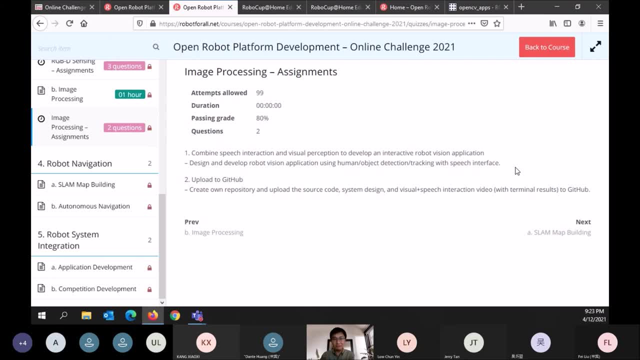 same person come into the frame, uh, the vision frame of the robot, then you can actually give the greeting, like, for example, like good morning, who and who? uh, and then you can say like what um services or what kind of things that you can provide. so, yeah, many things that you can do. 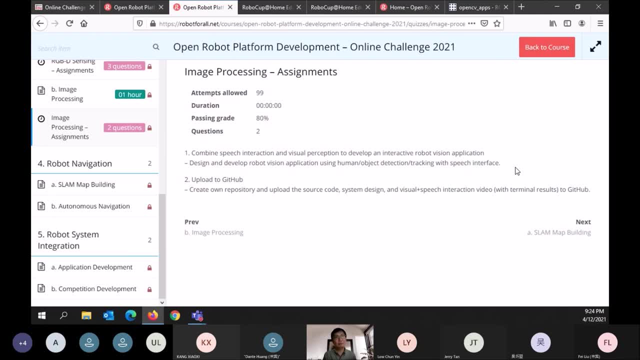 like for for this. so by combining whatever that you learned previous week and today, you can actually come up with a lot of scenario, and this kind of development are all inside, um, our scope of service robot development. okay, so you can. you can think of many, many things that. 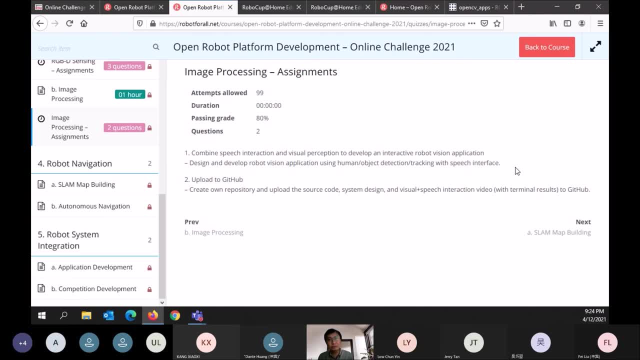 you can do so, hopefully, um, the things that we show you today, you can try to like figure out some way, uh, in order for you to design something interesting, uh, that you can do with just the minimum hardware that you have, and even you can do fancy with the. 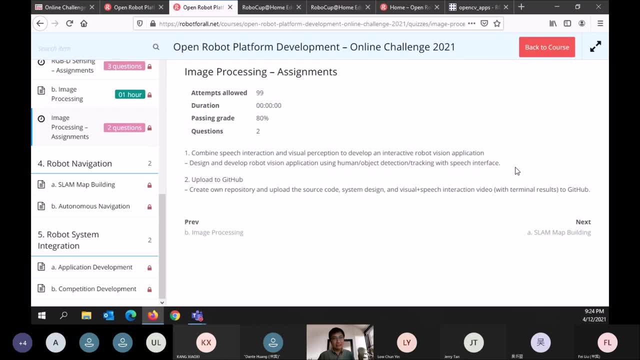 open post example, right, okay, so, hopefully, like, if you can do all this thing, you can upload the source code github and then we can- you can share with us, okay, or we can discuss, and this is something that, um, we look forward. right, okay, so i hope like i have. um, i explained everything for. 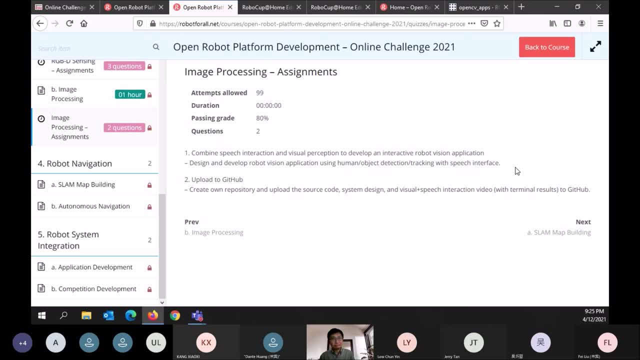 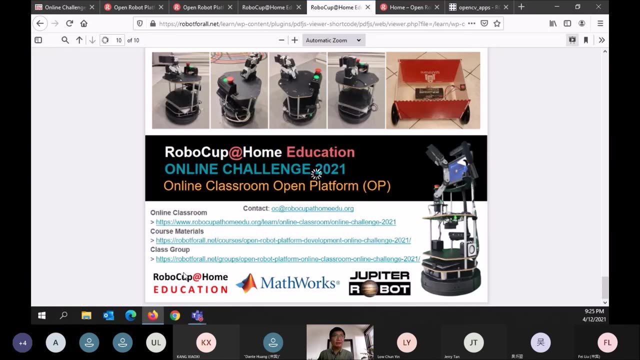 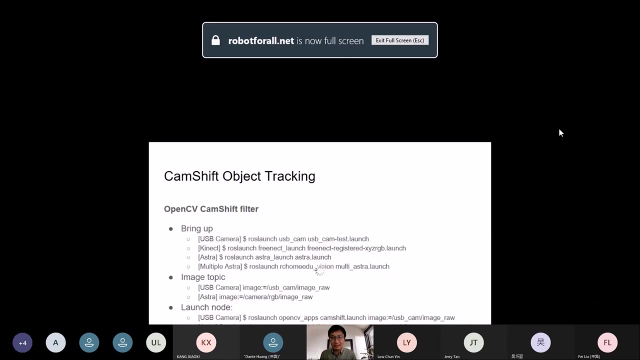 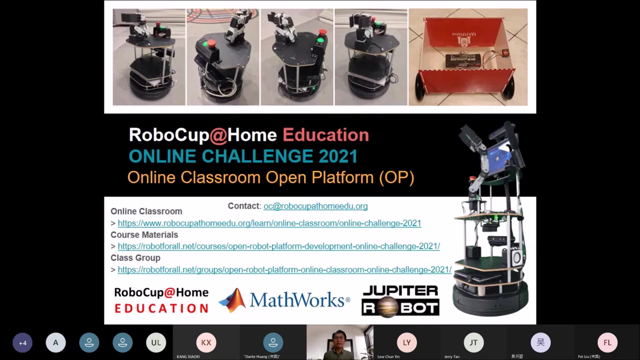 today. okay, so, oops, okay, so hope that, um, yeah, you can join the class group then and we can, we can discuss over there and so on. okay, so i would like to um close the session for today, uh, but since we already have about five minutes before our end of the session, so maybe please allow me to end this session. 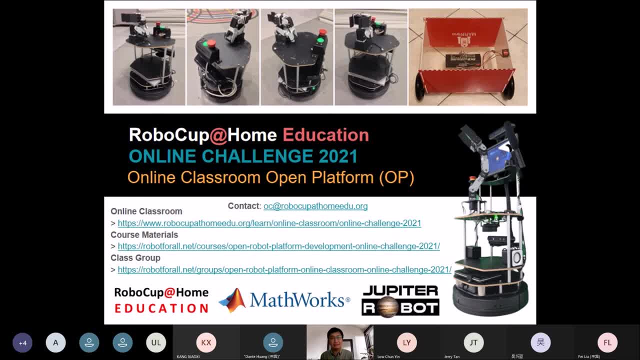 so that later on i can open up for our discussion. okay, because i i think like maybe it's more uh, relaxing if, let's say, we are not like recording the interaction. okay, so i will first close it. so please hold on and don't leave the the the meeting room. uh, we will do the. 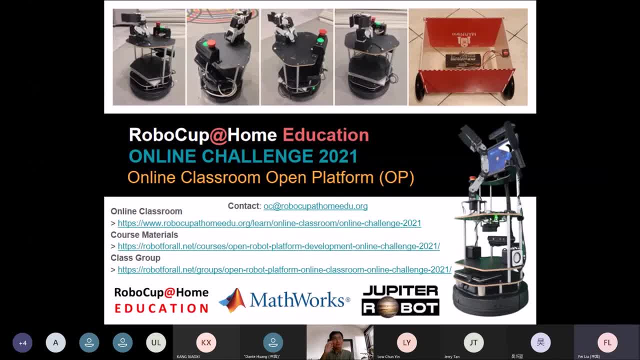 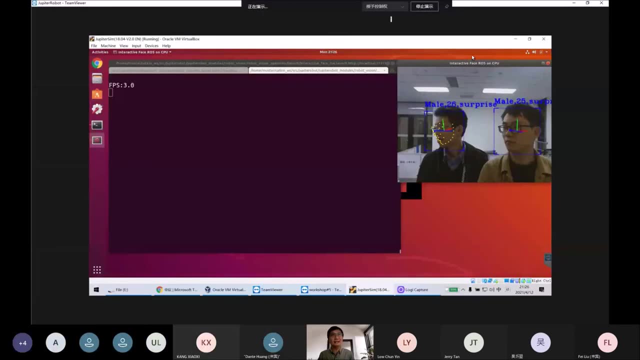 interaction after i stop the recording. okay, so with that i would like to. yes, could you please give me a few seconds of your shows, the interactive face result. okay, all right, so since, um, david already make it work, so maybe we can have a look. yeah, before we end the thing. all right, david, yep. 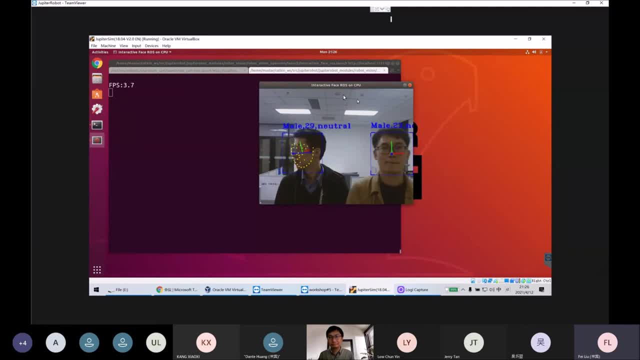 thank you. so now i will show you the result of the, a very interesting application, which means the interactive face, so you can see that the two face recognize uh. result here: uh, there is a yellow, yellow pointer around the face and it will show you the, uh, the, the male or female, and the. 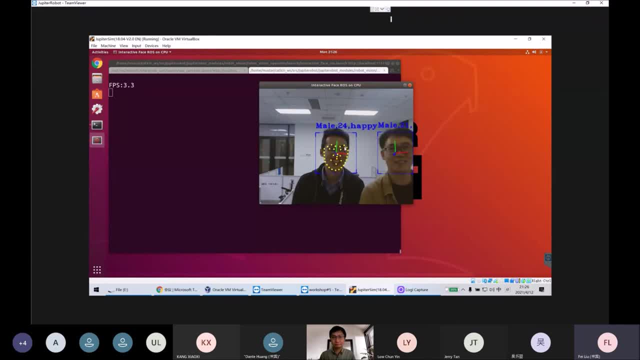 estimated age for this person and his uh, uh, his uh, his surprise, awesome, are surprised on each other's smile and said: maybe some uh, some, some, some- i don't know how to say expression, expression. okay, and there is also a three, uh a red, blue, green, uh, x. here you can show you the face. 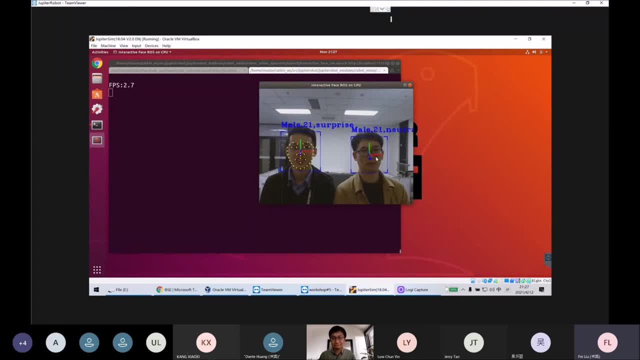 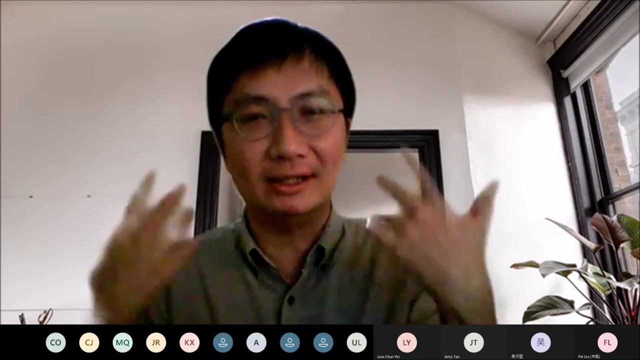 direct face, direct at the direction uh which the program can estimate: the face direction, to which angle or which position. so this is a very interesting uh interactive application. okay, thank you all right, thanks, david. thanks for the interesting um i'm sure. so this one will add to like one of um your tools that you can use, like just now when i say: 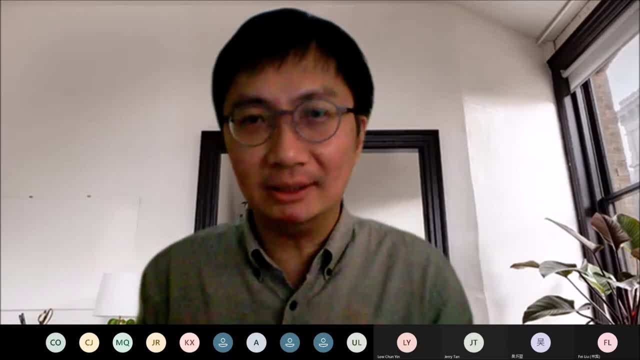 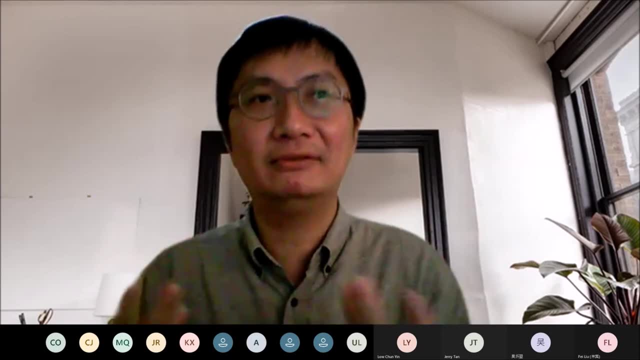 for the reception robot, so you can use some this to add up like: oh okay, so if it is a male or female, this over here will be your channel entity specific uh, somewhere around the unit, so you won't be able to see me on the video 때문에.